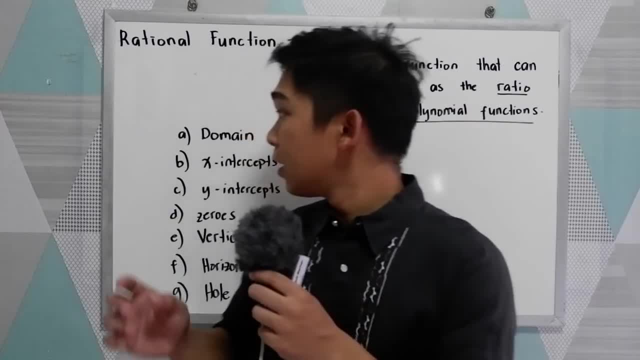 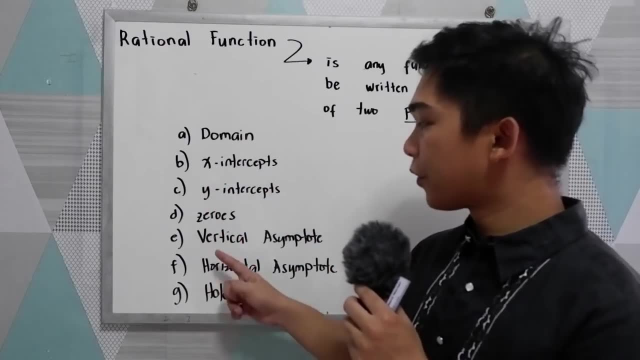 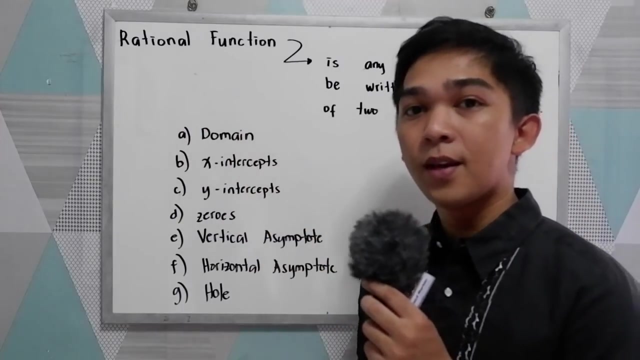 In this tutorial video, I will be teaching you how to get the domain, the x-intercepts, the y-intercepts, the zeros, the vertical asymptote, the horizontal asymptote and the whole of rational functions. Let us first define what is a rational function. 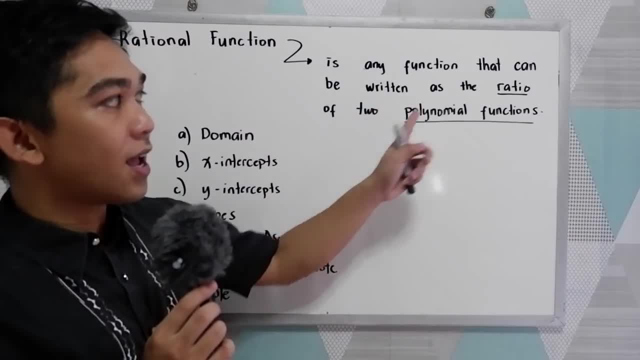 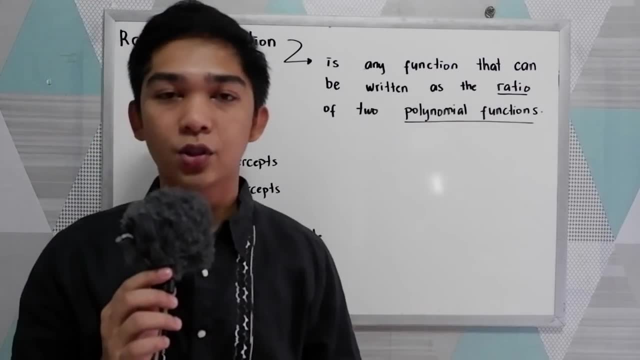 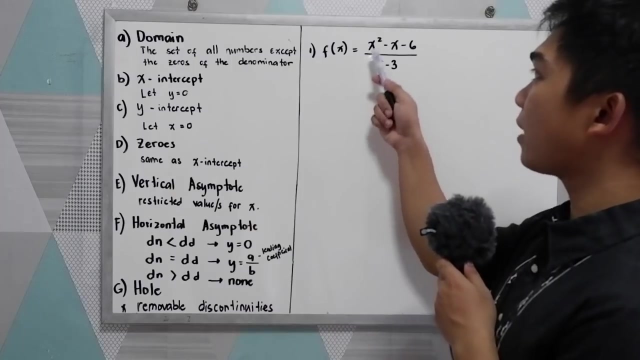 A rational function is any function that can be written as the ratio. So when we say ratio we have the numerator and denominator of two polynomial functions. Now let's have our problem number one. Let's say we have f of x is equal to x squared minus x minus six, all over x minus three. 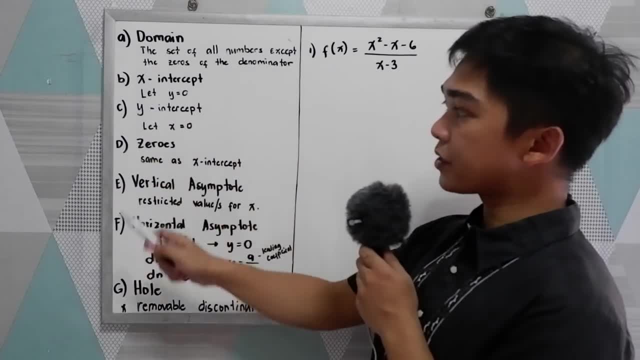 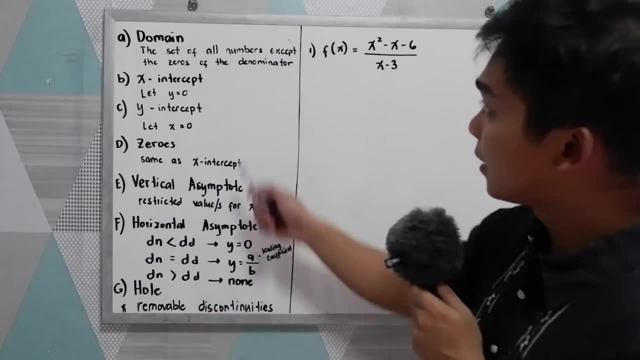 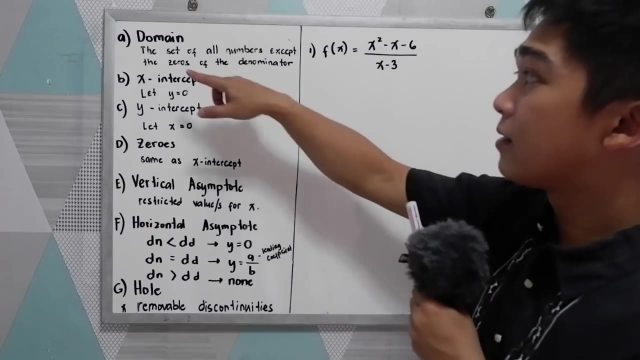 We're going to find the domain, the x-intercept, y-intercept, zeros, the vertical asymptote, horizontal asymptote and the whole. If you notice, we have a guide in every item, So for the domain. so let's find first the domain. The domain is the set of all numbers except. 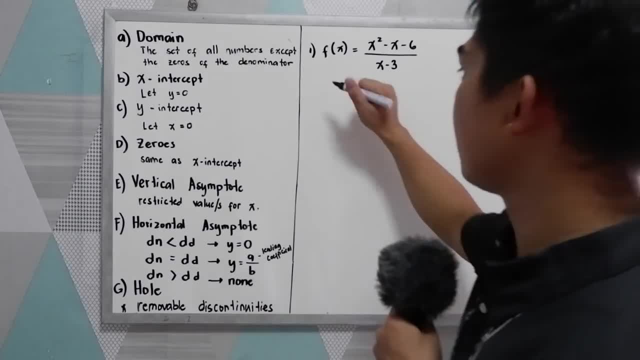 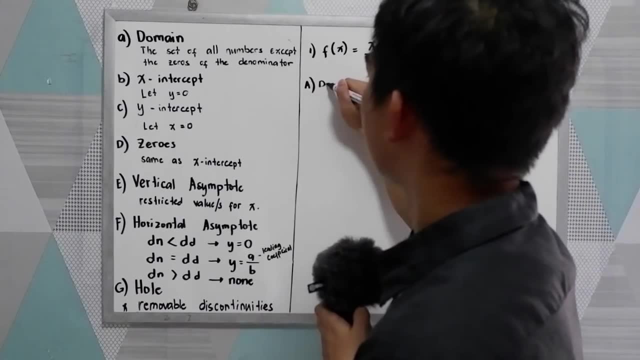 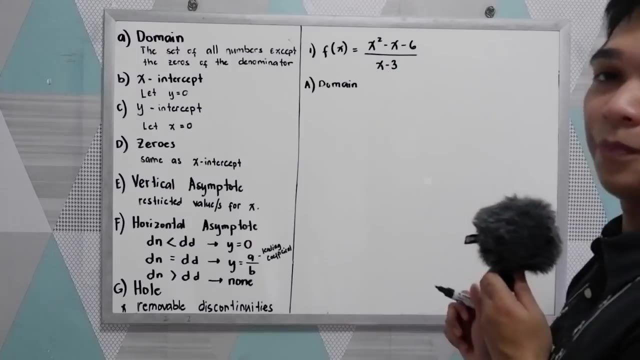 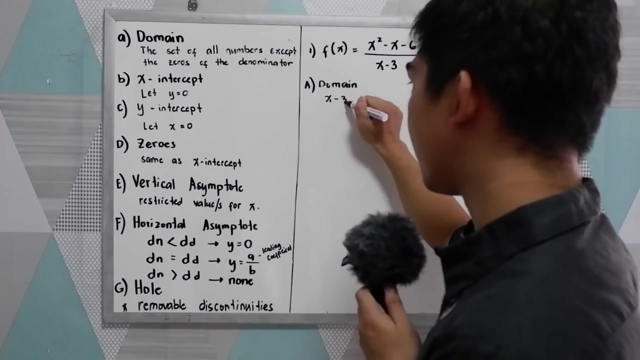 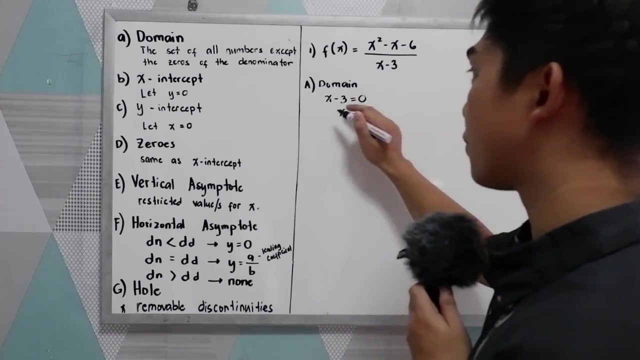 the zeros of the denominator. So for the domain, let's say a domain, Find the zeros of our denominator. So our denominator here is x minus three. So copy: x minus three Just equate to zero. So solve for x. So we have x is equal to positive three. 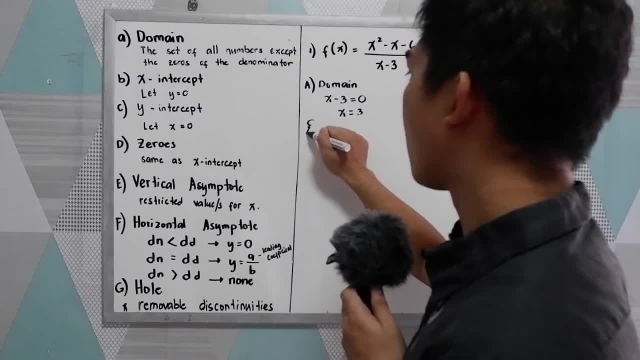 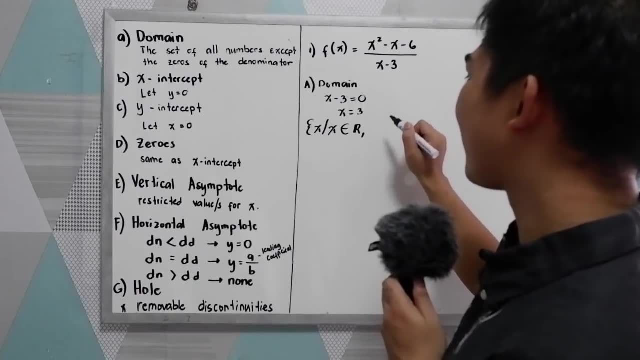 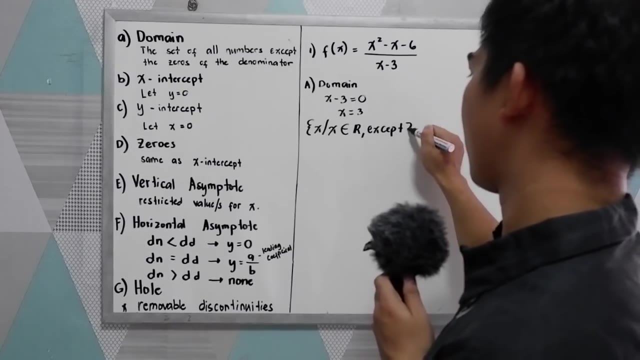 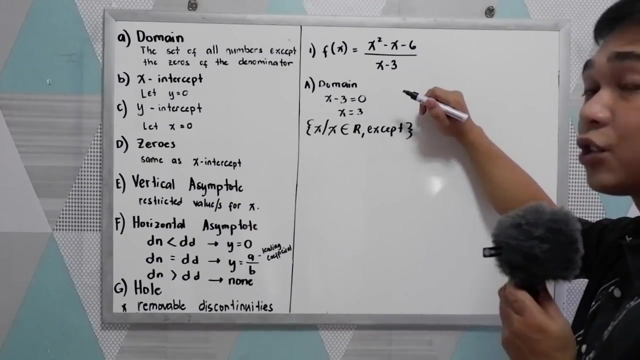 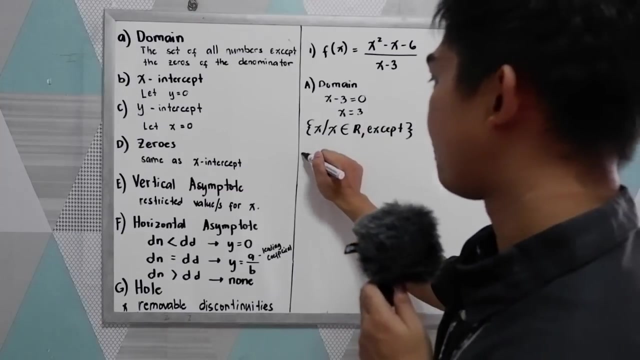 So our domain is x, such that x is an element of real numbers except three. Or simply just get the value for x to make our rational function undefined. So get our denominator, then equate to zero, Then letter b, x-intercept. So we have. we have it here in the tenth digit. here Then we have the domain: Now no. Or just to make our writer function undefined, So get our denominator then equate to zero, Then letter b: x-intercept. 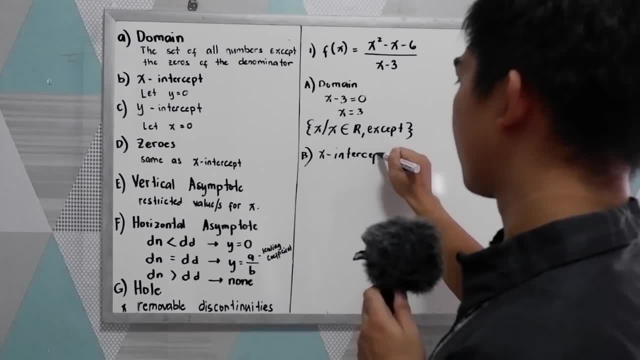 So just find the spacing of x basketball. So go there. We're going to find that there. Tell us the shape of your picture, That those oben so 점 um, to determine that we draw the circle right there. 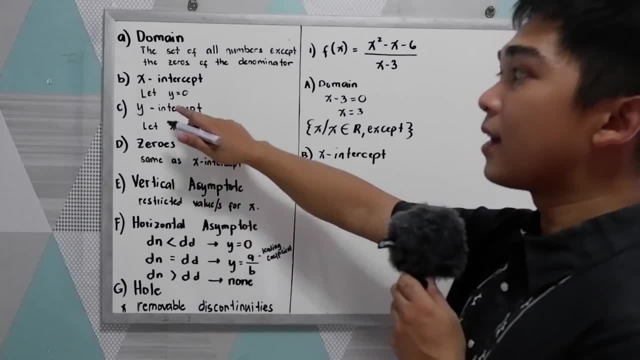 Let's go to the circle, And then we must erstenize to complete our нашей ich, that is oureration. Uh, y is equal to 0. Again, we have 1. the X intercept: let Y be equal to 0. so f of X, that is, stands for our Y, so we. 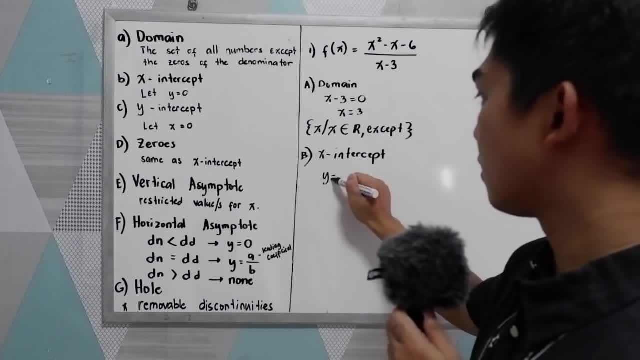 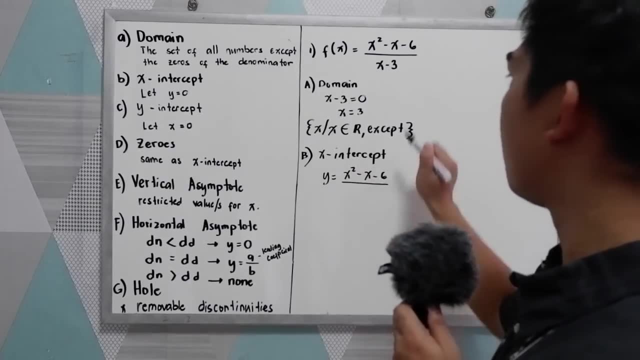 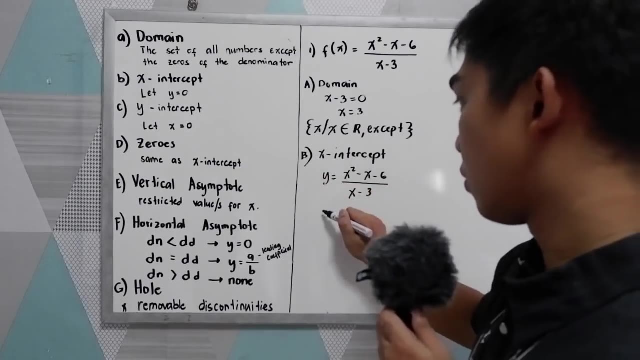 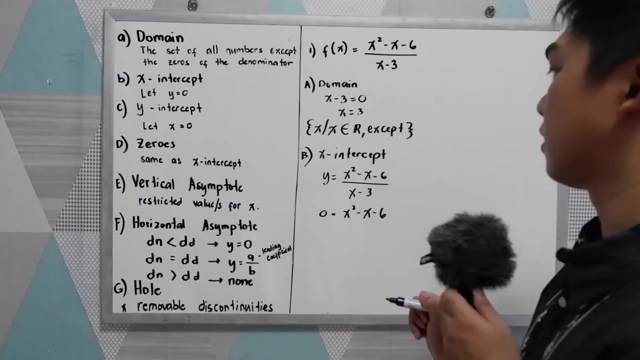 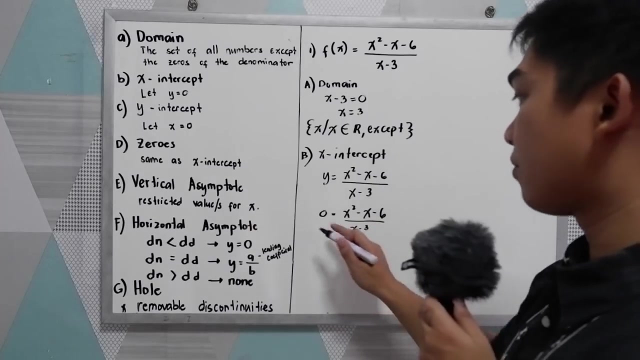 have Y. f of X is our Y. then we have X squared minus X minus 6, all over X minus 3. let Y be equal to 0, so Y be 0. and we have now X squared minus X minus 6 all over X minus 3. cross multiply so we have 0 times X minus 3. that will become 0 is. 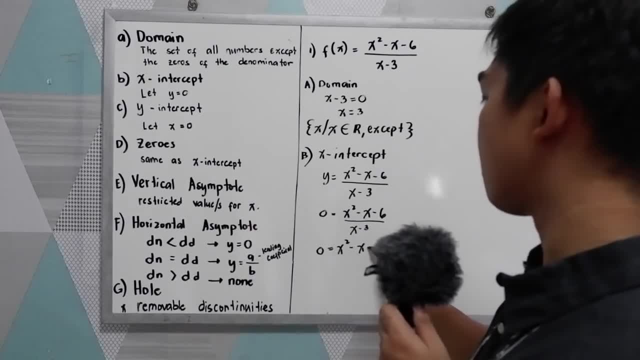 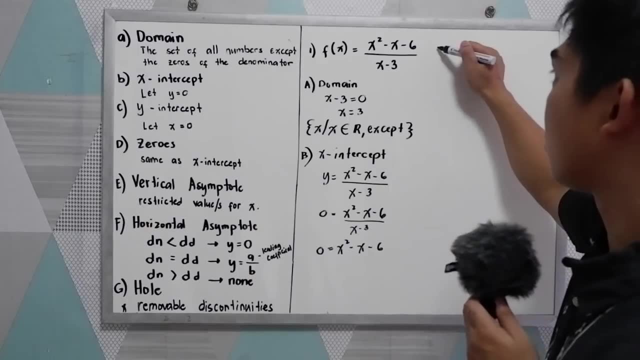 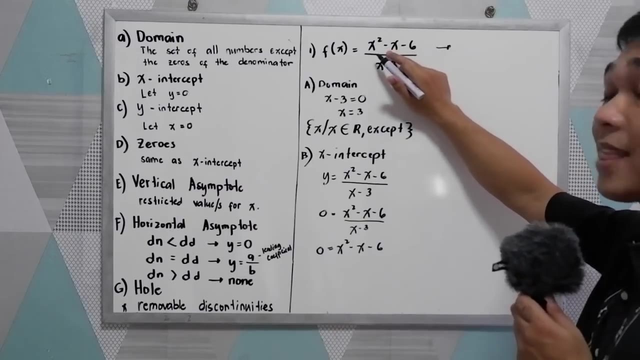 equal to X squared minus X minus 6. now let us factor X squared minus X minus 6. okay, to get the factor, get the product of negative negative 6, the sum must be negative 1. so factoring the three poisoned outs, factoring X and X. 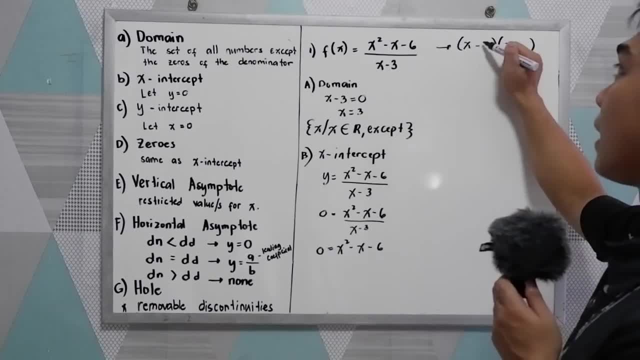 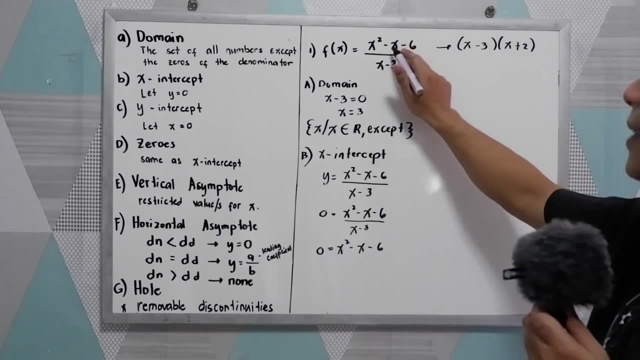 factors of negative 6. we have negative 3 and positive 2. let us check: negative 3 times positive: 2, that is negative 6. negative 3 plus 2 that is negative 2.. 1 or simply negative X here. so this function is just equal to X minus 3. 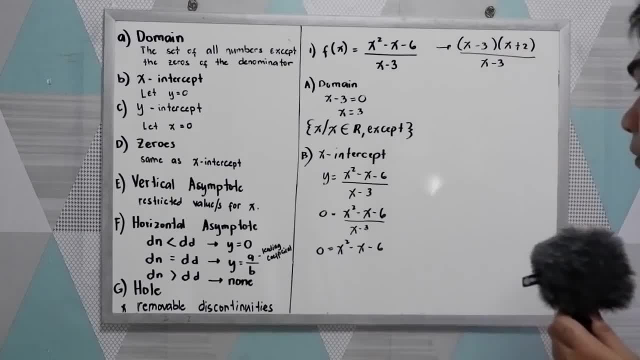 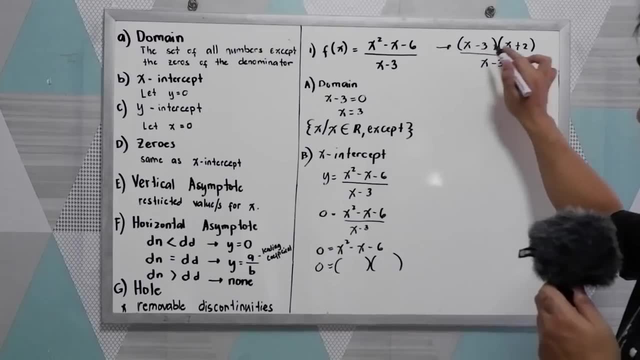 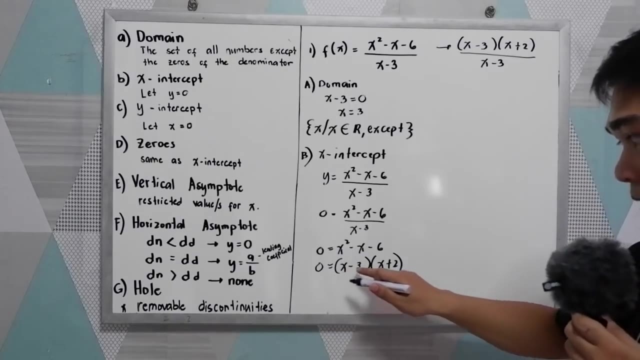 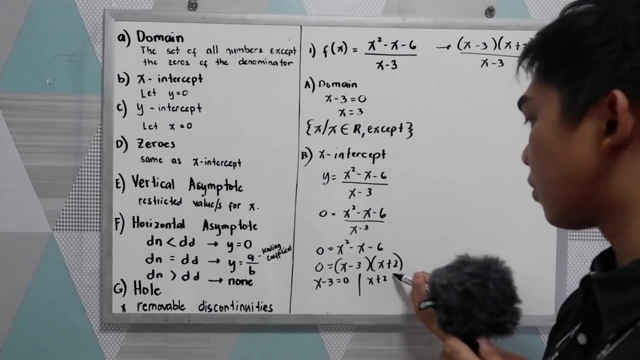 times X plus 2, all over X minus 3. okay, let us write here: go back in letter B. 0 is equal to just copy the factored form X minus 3 and X plus 2 now equate to 0. so we have X minus 3 is equal to 0 and X plus 2 is equal to 0. so for X, so X is: 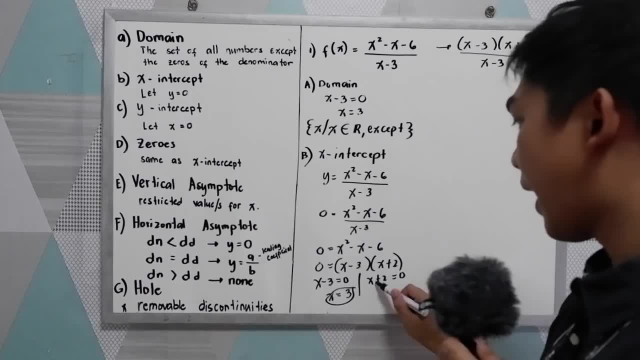 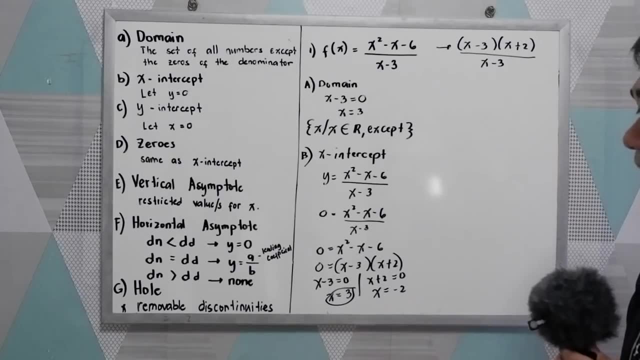 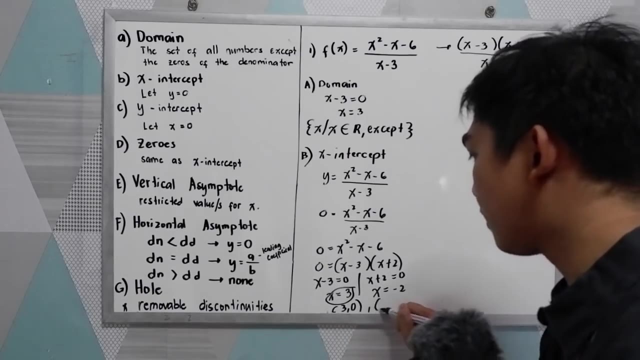 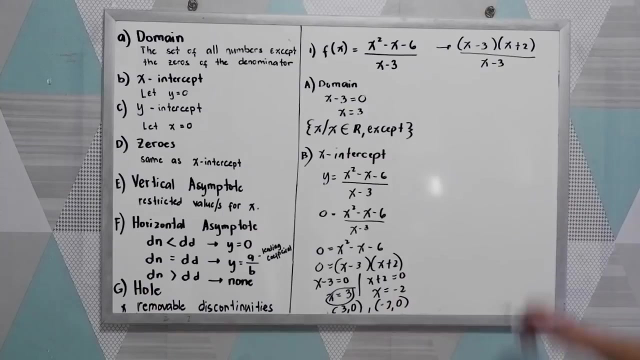 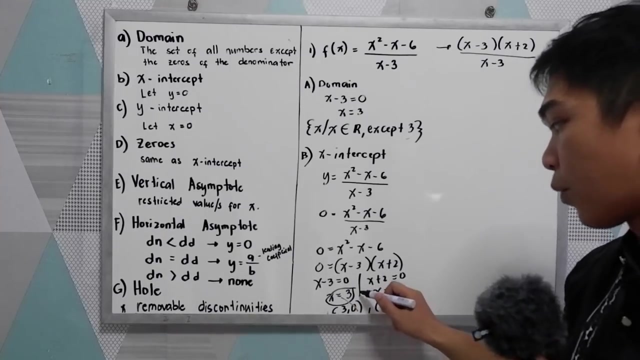 equal to positive 3, and here X is equal to negative 2. so we have 2 X intercepts, we have 3: 0 and negative 2: 0. but take a look in our domain that our X must not be equal to 3, so we're just going to consider negative 2: 0. so our X intercept is: 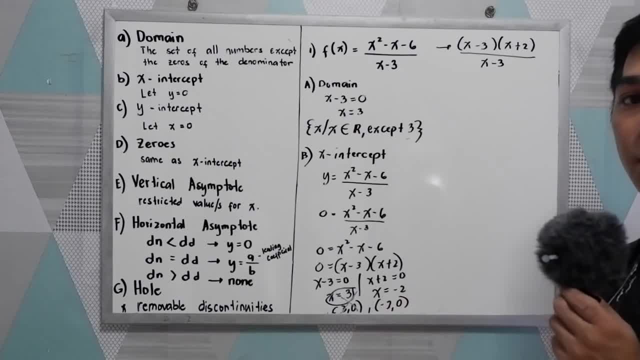 negative 2, 0.. Where did we get 0? that is the value of our Y, so our 271 00007. let's have a short review. our x-intercept is a point. that means it must contain our abscissa and ordinate. so our x here is negative 2, then y: 0. now. 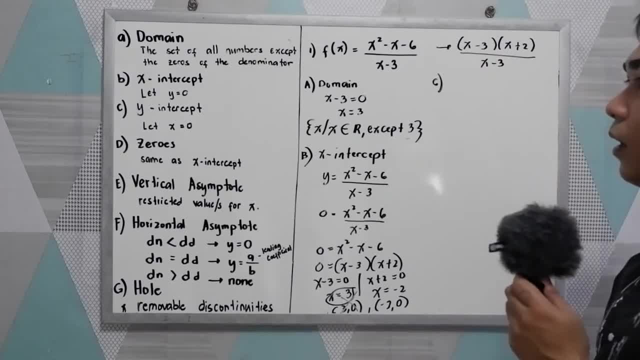 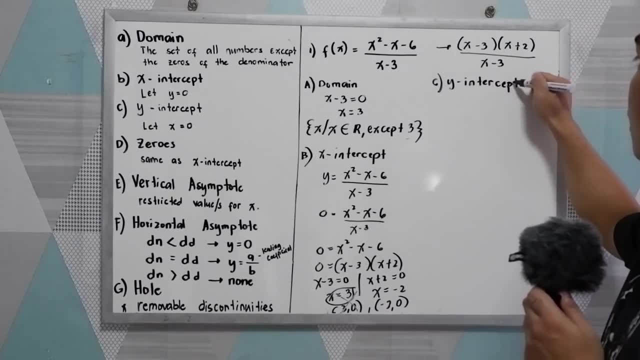 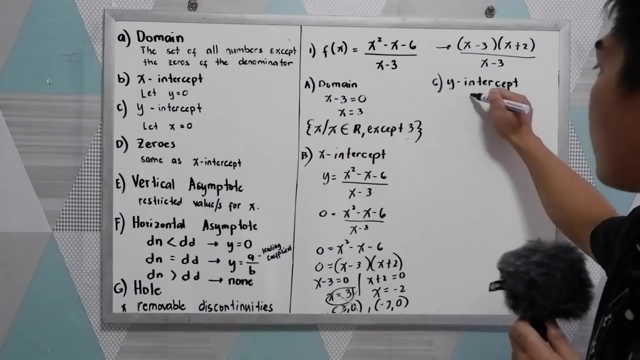 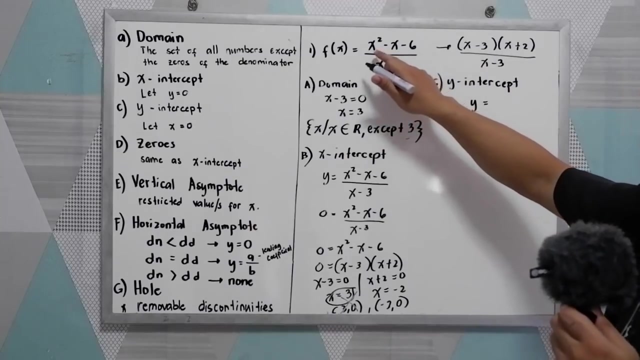 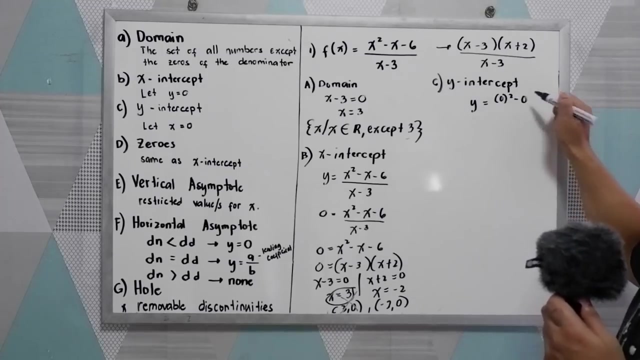 let us see y-intercept, y-intercept for the y-intercept: let x be equal to 0, so we have. let x be equal to 0, so y is equal to the substitute our x to 0, so we have 0 squared minus 0. change x to 0 minus 6, all over 0 minus 3, now we have. 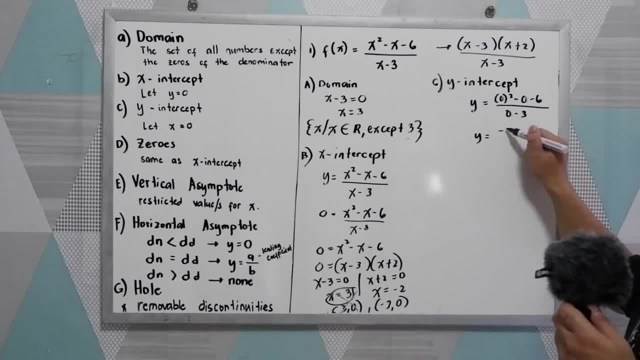 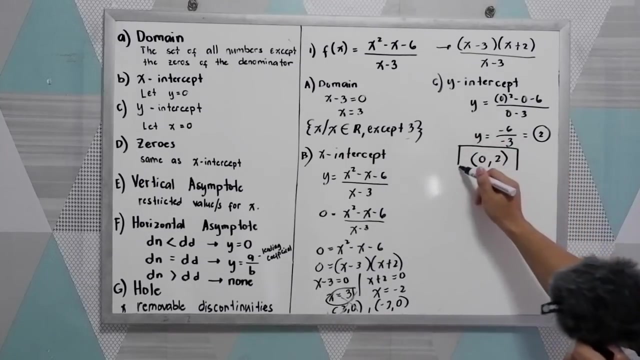 that is 0 minus 0, that is 0 minus 6. so negative 6 all over 0 minus 3. negative 3. negative 6 divided by negative 3, that is positive 2. so our y-intercept is: our x is 0. so we have 0 positive 2. this will be our x-intercept. 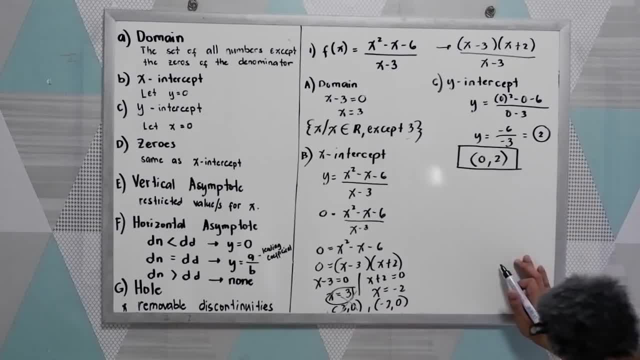 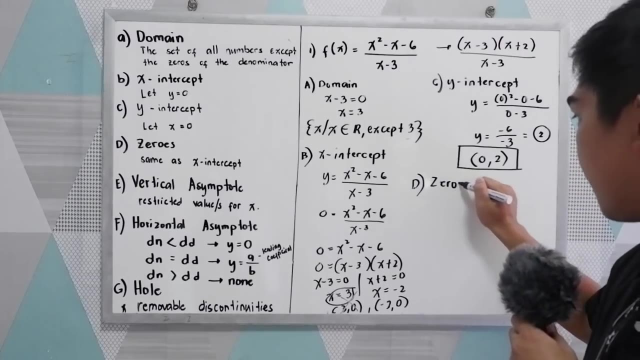 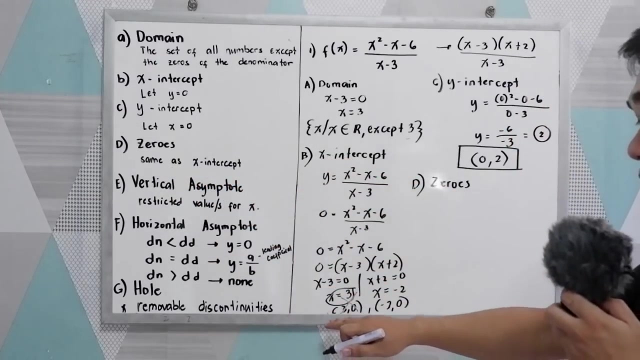 okay, or y-intercept, a yz equal to do left, left or D. now let's have the zeros of our rationale function, zeros in our guide. this is the same as our x-intercept. so let there be x-intercept. we have our solution here and we're going to find the value for. 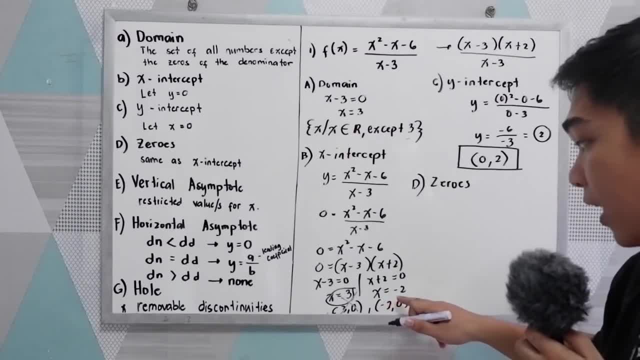 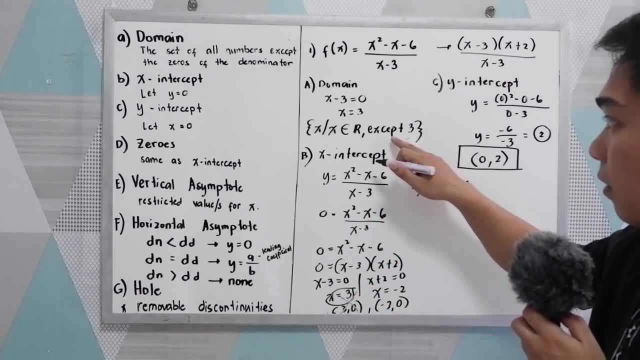 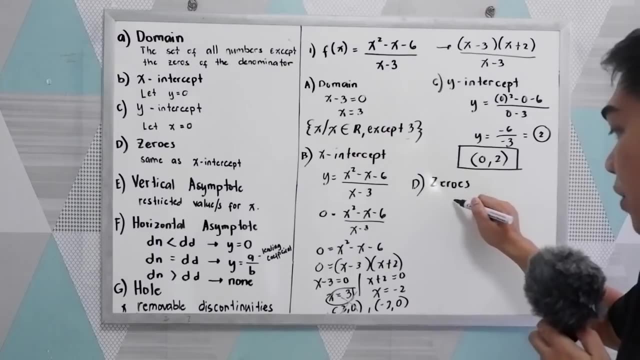 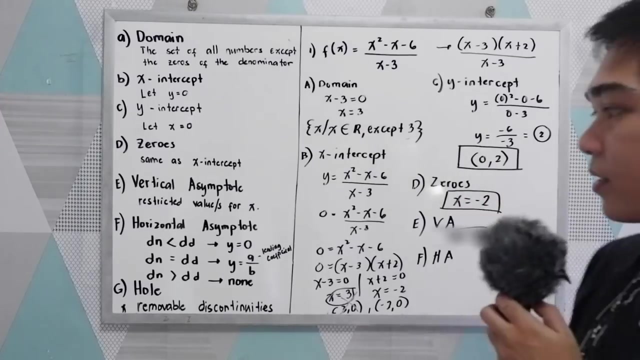 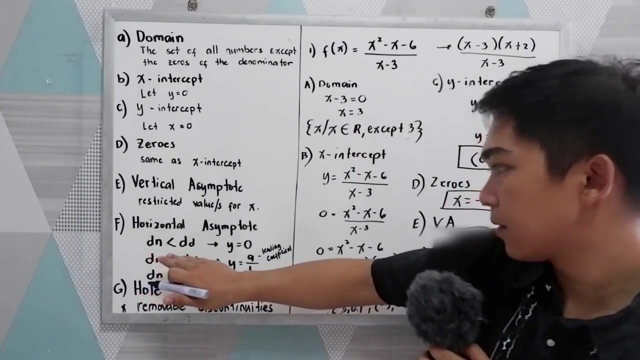 our X is equal to negative 2 and positive 3. but take a look. but take a look in our domain: our restricted value for x is 3, so x is a restricted value. for our zeros, x is equal to negative. we discussed here because this is a crucial part. let's have our first condition. 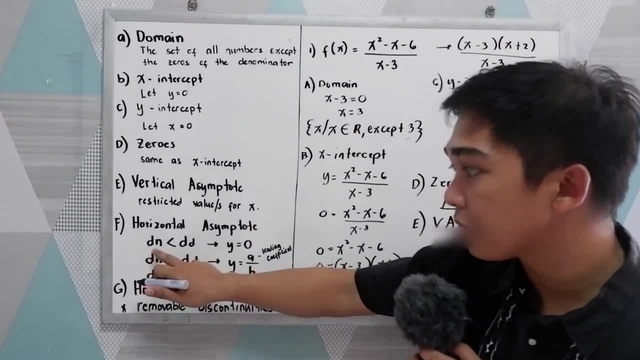 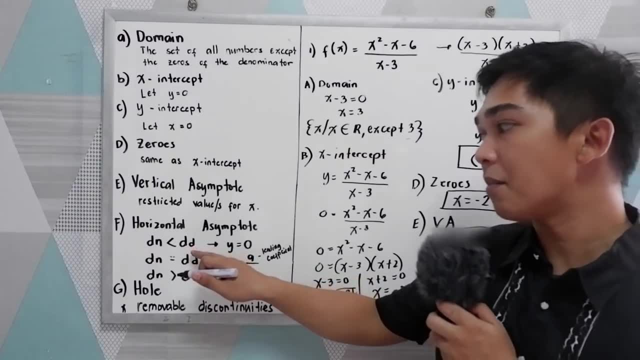 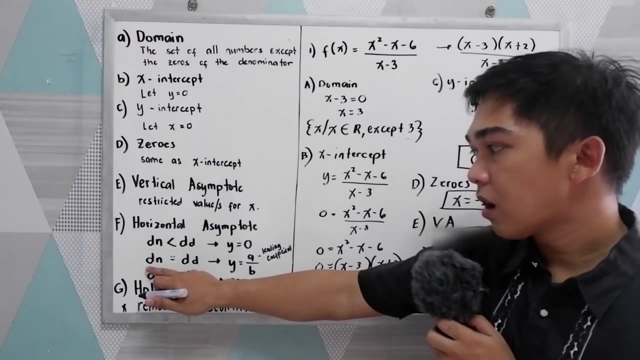 d here stands for the degree, if the degree of the numerator and stands for the numerator. if the degree of the numerator is less than the degree of the denominator, our y is equal to zero in If the degree of the numerator is equal to the degree of the denominator. 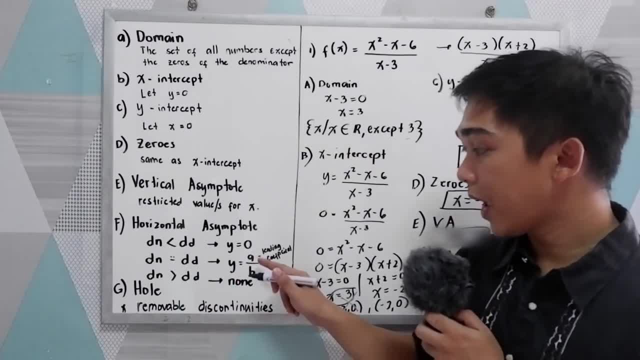 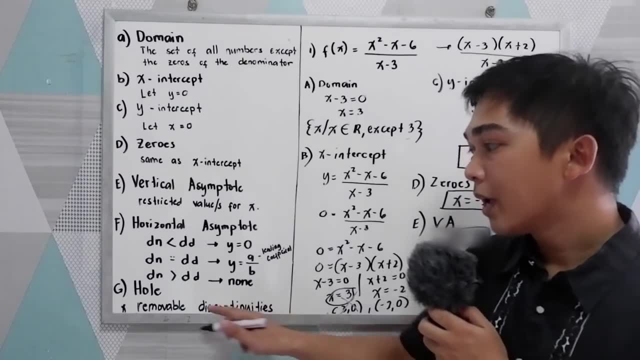 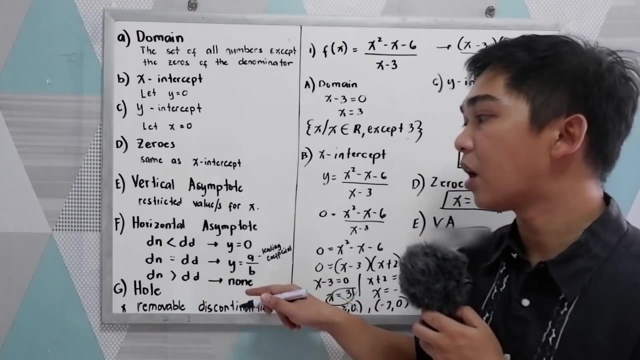 we're going to use a over b, where a is our leading coefficient in the numerator and b is the leading coefficient in the denominator, And if the degree of the numerator is greater than the degree of the denominator, we don't have a horizontal asset. 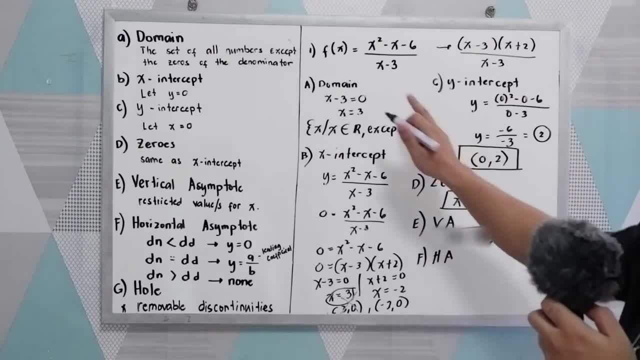 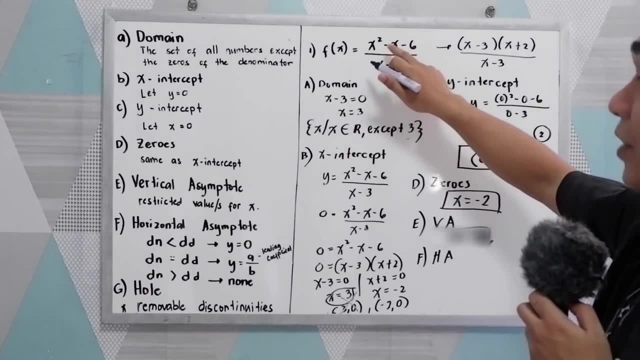 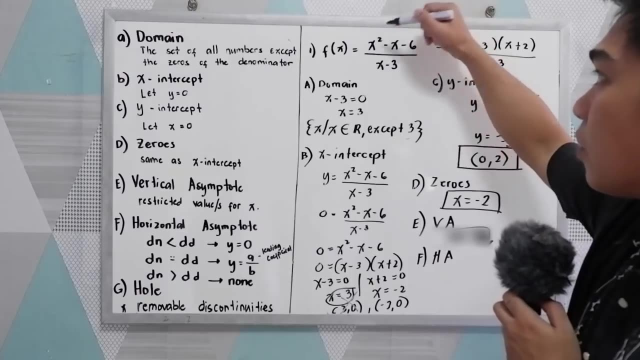 Now we're studying our given. The degree of our numerator is greater than the denominator In our numerator. we have here our quadratic, so our degree in the numerator is two and in our denominator. that is a linear function, so one. 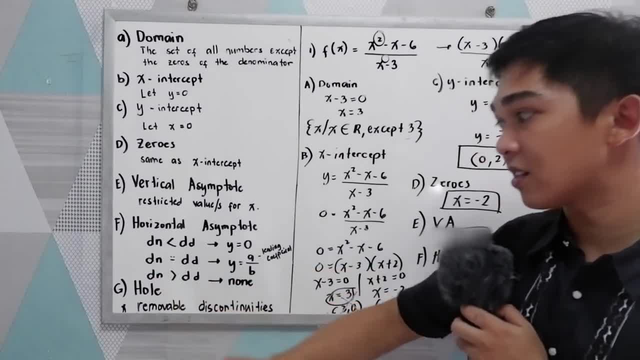 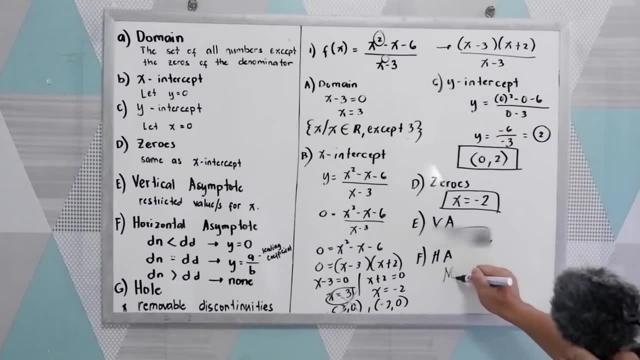 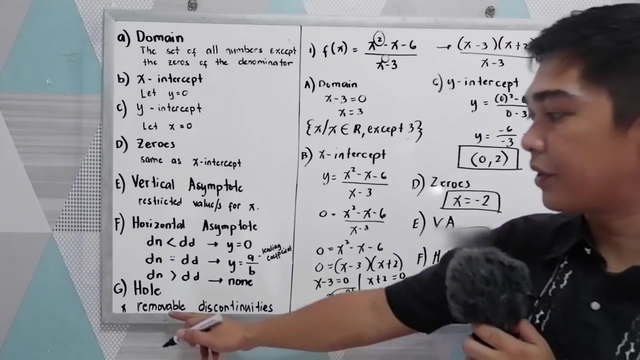 So the degree of the numerator is greater than the degree of our denominator. so, horizontal asset. in this case, we don't have none. There's no horizontal asset. Now let's have g, the hole. Okay, hole is also known as the removable discontinuities. 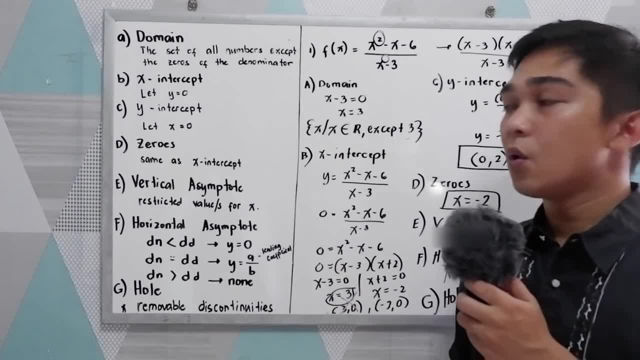 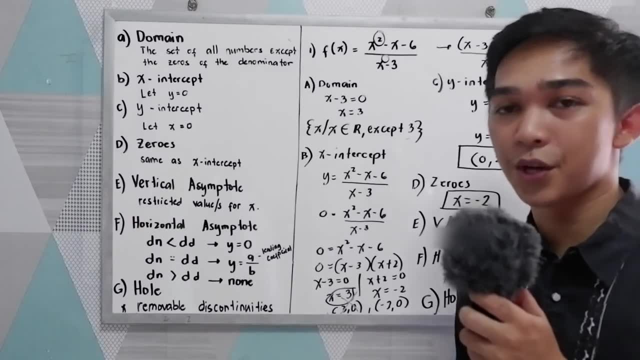 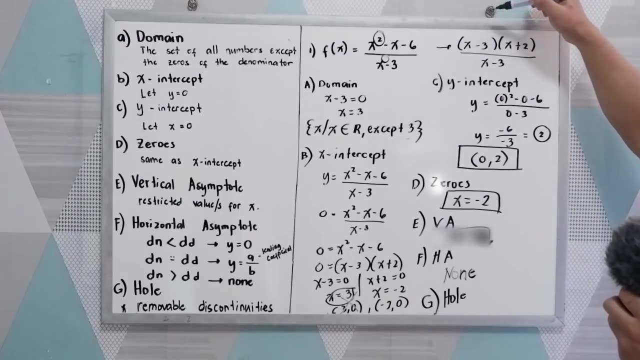 So these are the values or the inputs that causes our numerator and denominator be 0. So in this case, notice that we have a common factor in our numerator and in the denominator. So these are the discontinuity of our function. So get the. 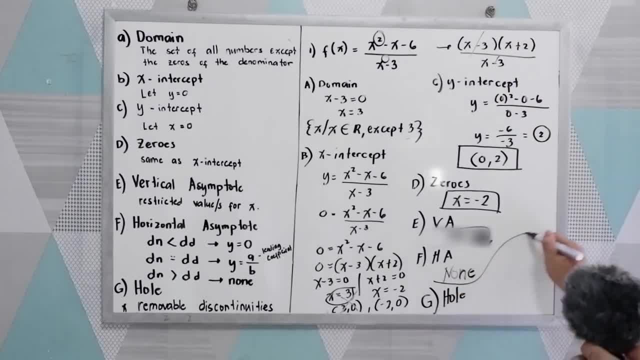 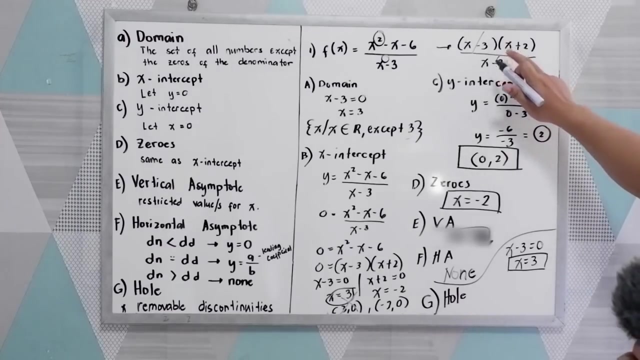 common factor for the whole. We have x minus 3 is equal to 0. That is the common factor. So find the value for x, So x is equal to 3.. Now we have our abscissa, or our x, To find our y. get the remaining factor in our numerator, which is x plus 2.. 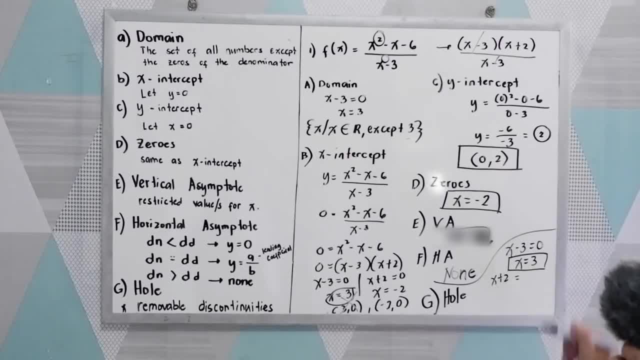 So x plus 2.. Now substitute the value of our x, which is 3.. So we have 3 plus 2.. Now we have 3 plus 2.. We have 5.. Now the coordinate of our whole is x is 3.. Then this will be the. 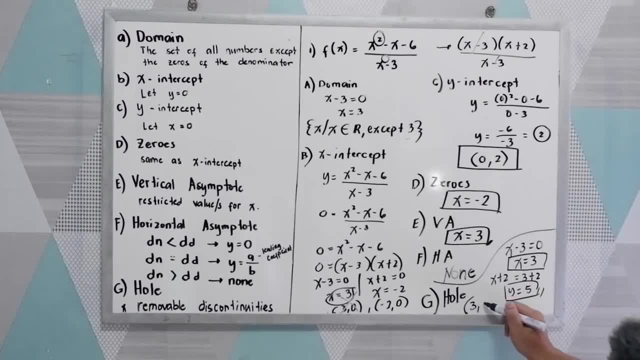 value of our y, 3 comma 5.. That would be the discontinuities of our rational function, 3 comma 5.. This is the whole. Again, if we have a common factor in the numerator and denominator, get the common factor then equate to 0, then solve for x And after. 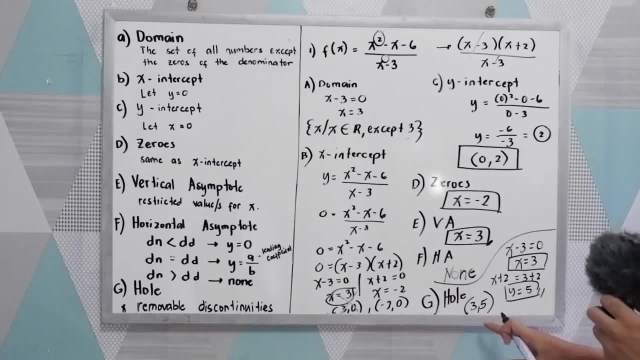 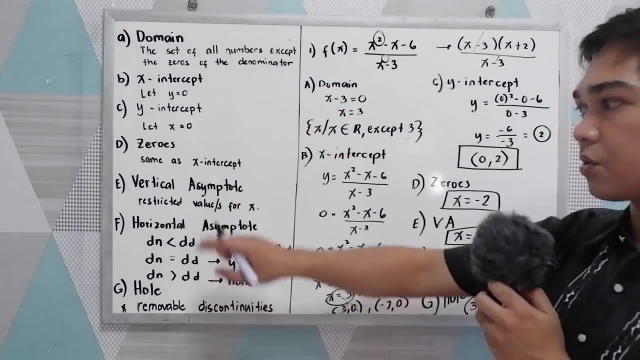 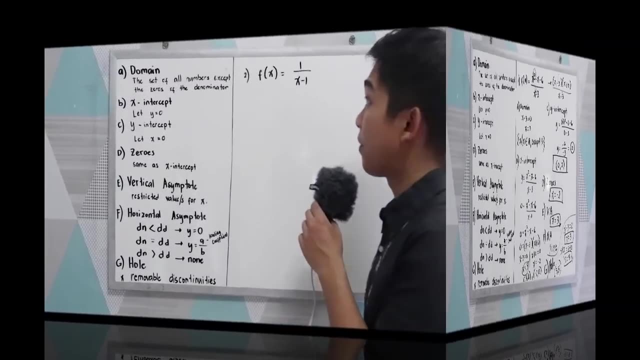 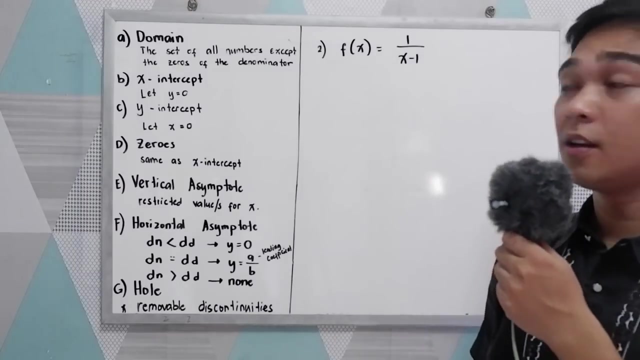 that substitute to get our organic. Okay, That is, on how to find the domain, x intercept, y intercept, the zeros, vertical asymptote, horizontal asymptote and whole. Let's have our second example. Now. let's have our second example. f of x is equal to 1 over x minus 1.. Let us find: 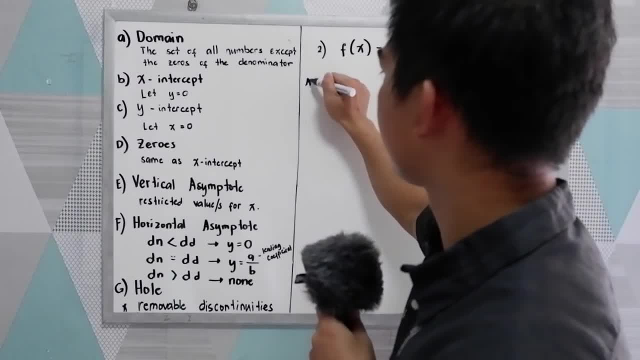 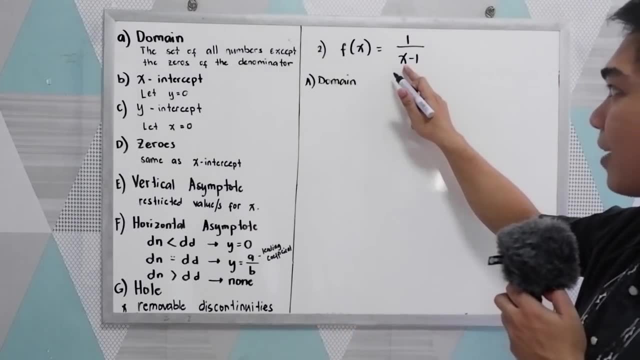 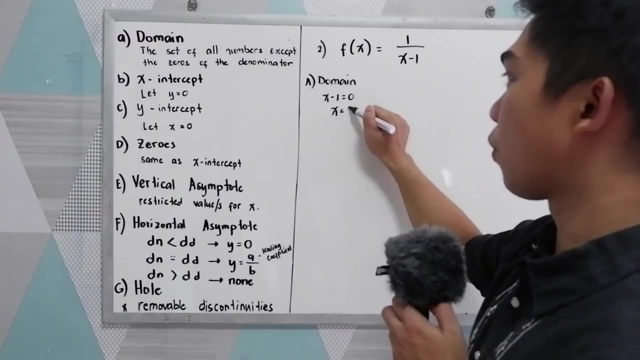 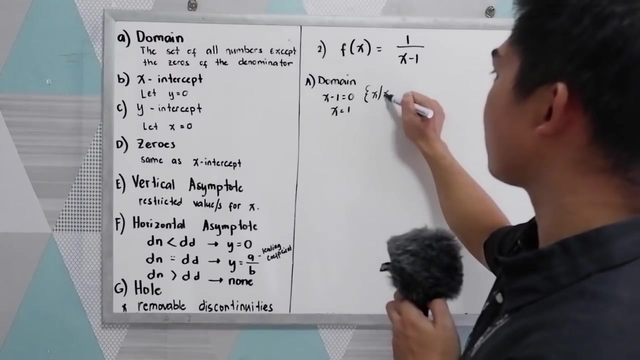 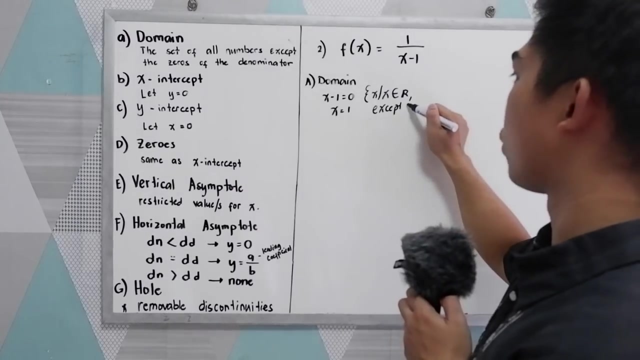 the domain, So letter a domain. So get the denominator x minus 1, equate to 0. So x is equal to 1. So our domain is x, such that x is an element of real numbers except positive 1.. 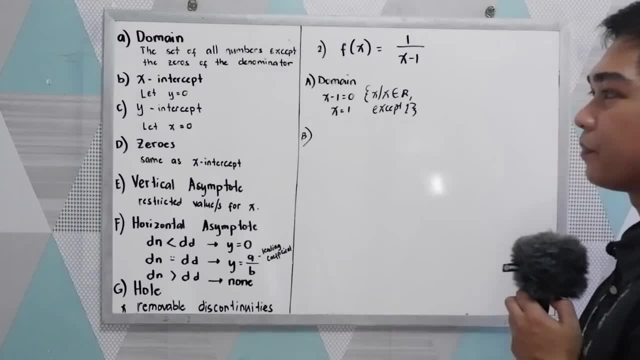 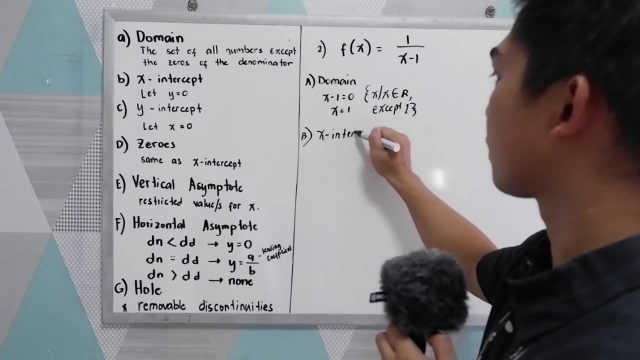 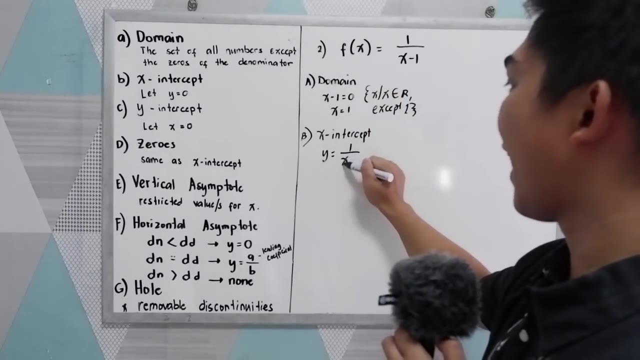 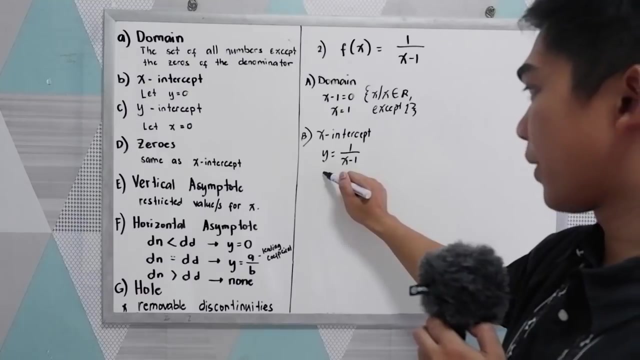 b, the x-intercept. For the x-intercept, let y be equal to 0. So x-intercept. so y is equal to 1 over x minus 1.. Again, f of x is the same as our y. so let y be equal to 0.. 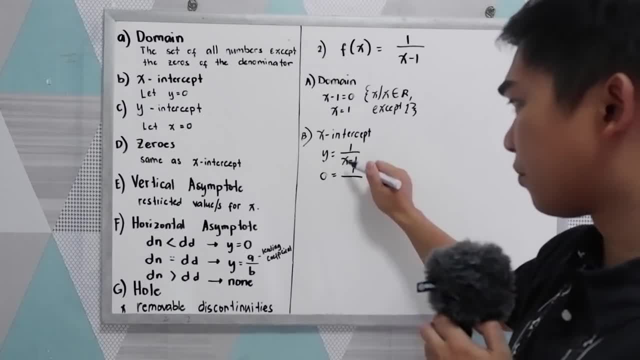 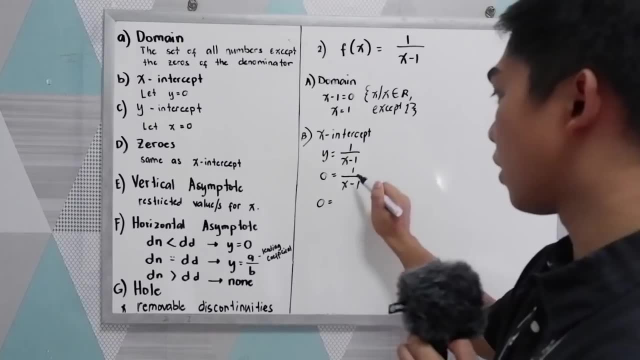 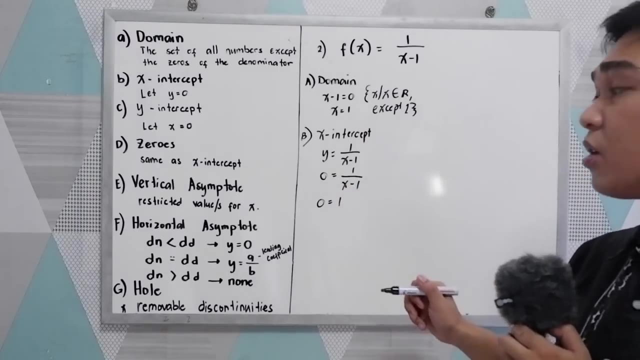 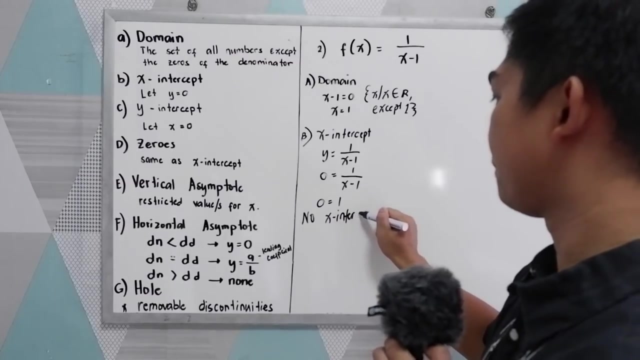 So we have: 0 is equal to 1 over x minus 1.. Cross-multiply so we have: 0 is equal to 1.. Notice that we don't have a 1.. I'm calling for x because 0 times x minus 1 is 0, so that means we don't have no x-intercept. 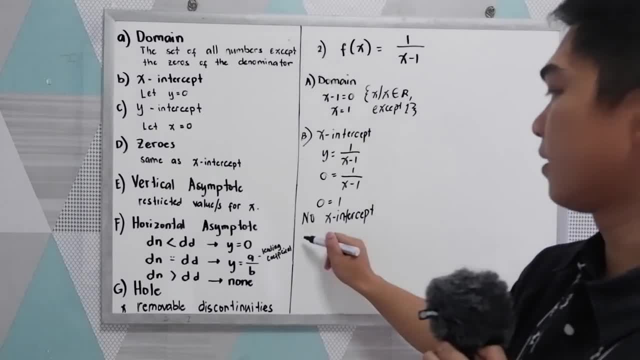 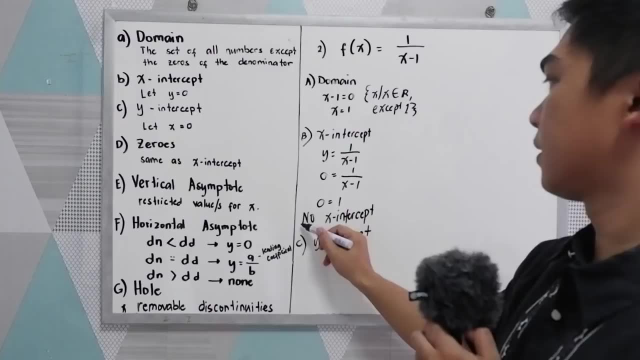 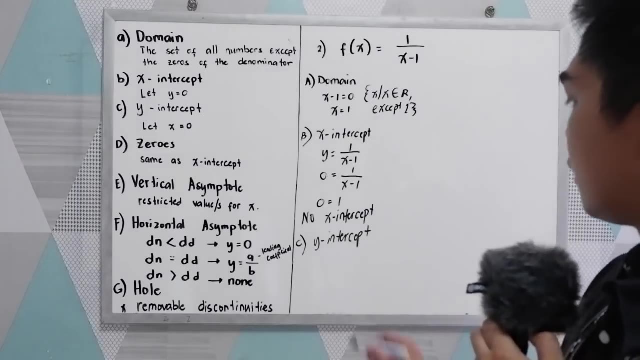 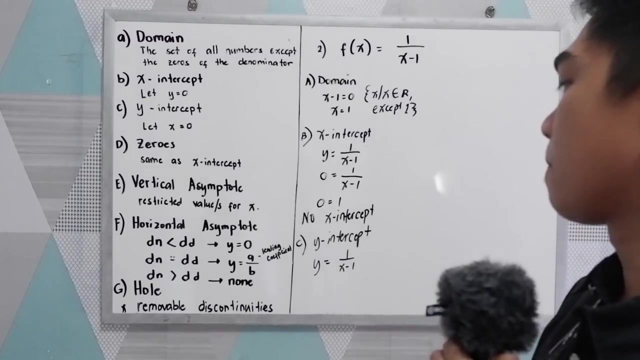 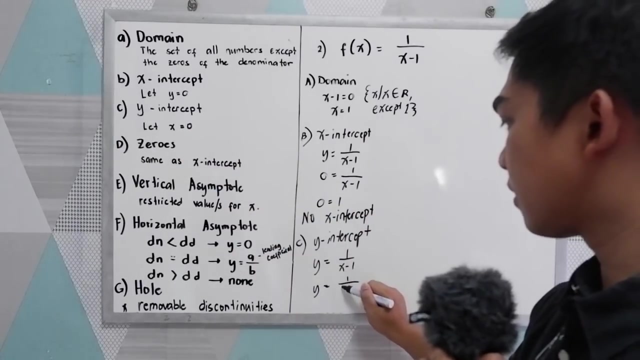 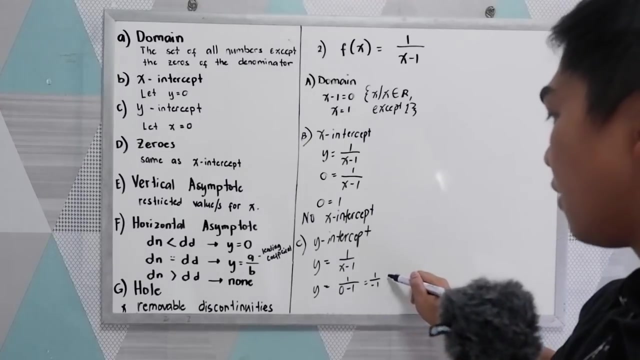 or simply none For the x-intercept: none Letter c: y-intercept. For the y-intercept, let x be equal to 0.. Okay, So we have y is equal to 1 minus x minus 1.. Let x be 0,. so we have y is equal to 1 over 0 minus 1, and that is 1 over negative 1.. 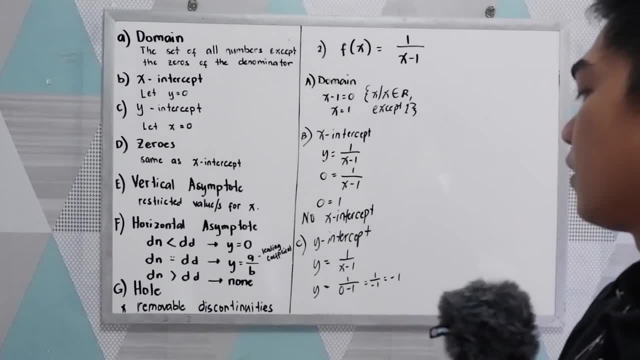 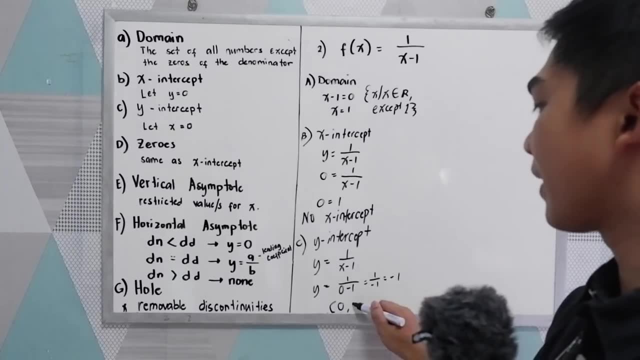 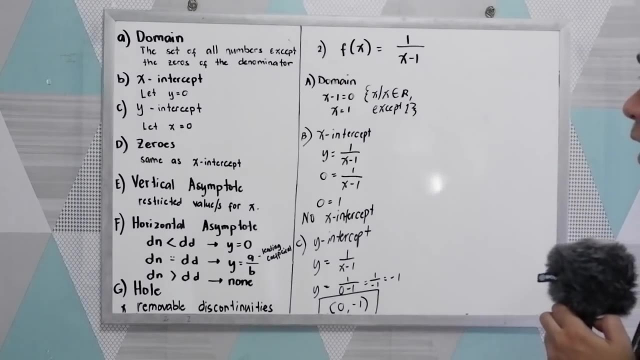 Therefore, y is equal to negative 1.. So our y-intercept is 0.. Okay, So our y-intercept is 0, negative 1.. That is our y-intercept. And for the 0's letter, d, 0 is the same as the x-intercept, so we don't have x-intercept. 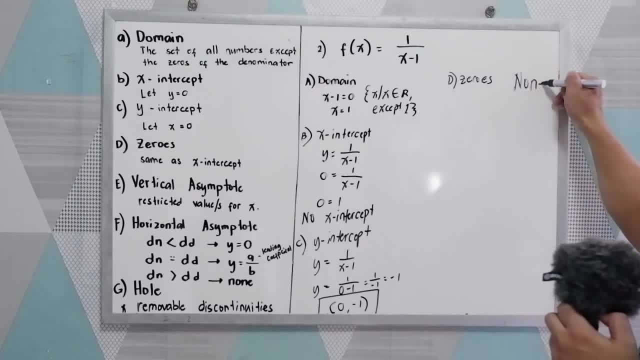 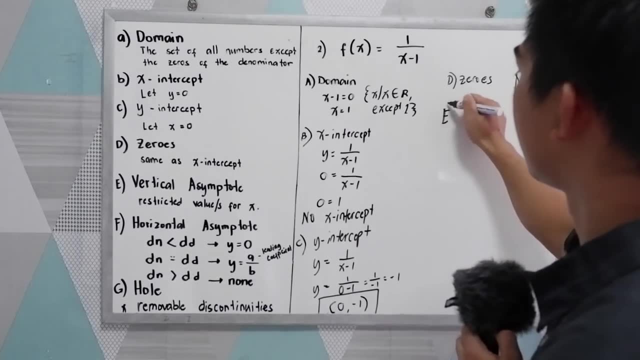 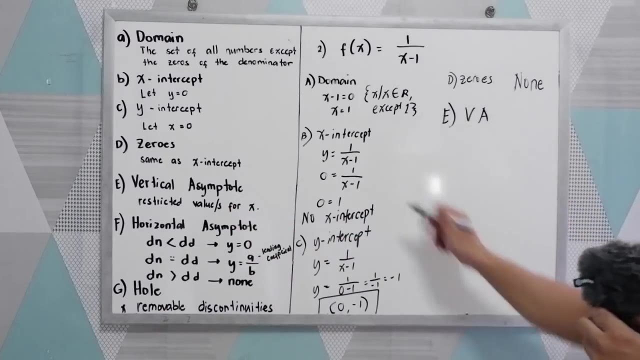 So 0 is 9.. Okay, And for the vertical asymptote, letter E, these are the restricted values for x vertical asymptote According to our domain, x, such that x is an element of real numbers except 1.. 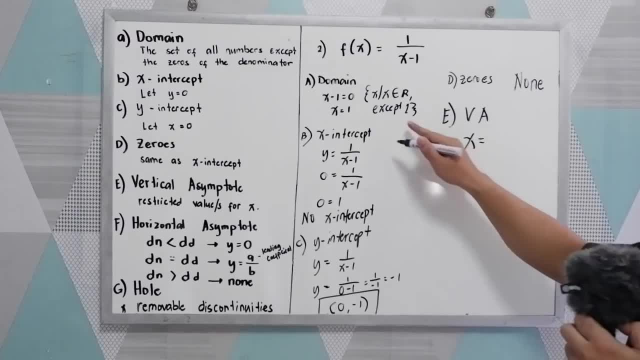 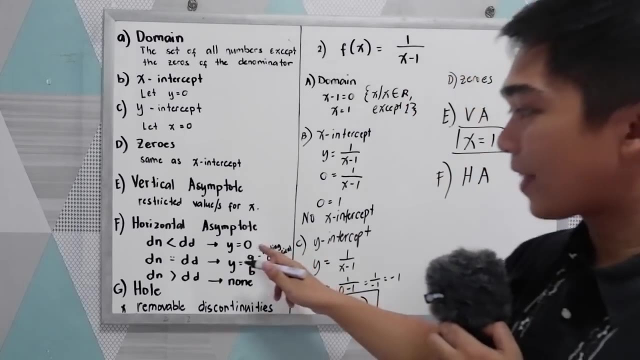 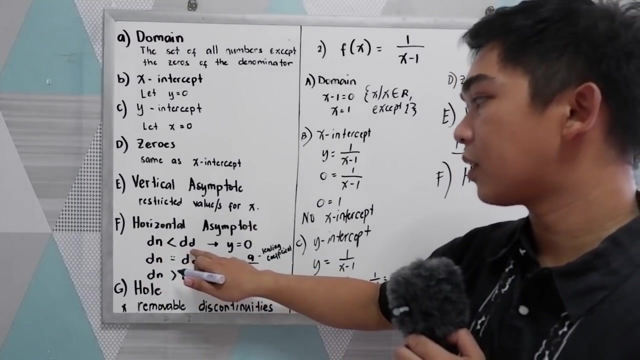 So vertical asymptote x is equal to 1.. Letter F: horizontal asymptote 1 over x minus 1.. So study our condition. if the degree of the numerator is less than the degree of the denominator, our horizontal asymptote is: y is equal to 0.. 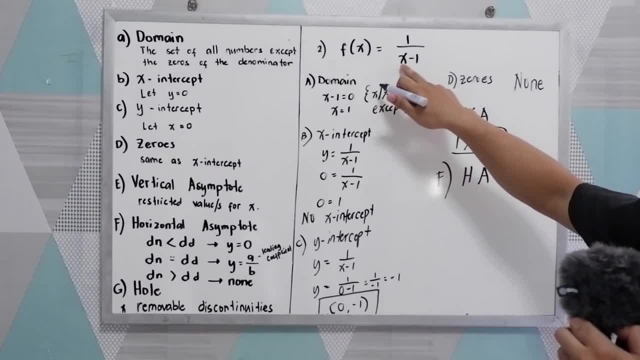 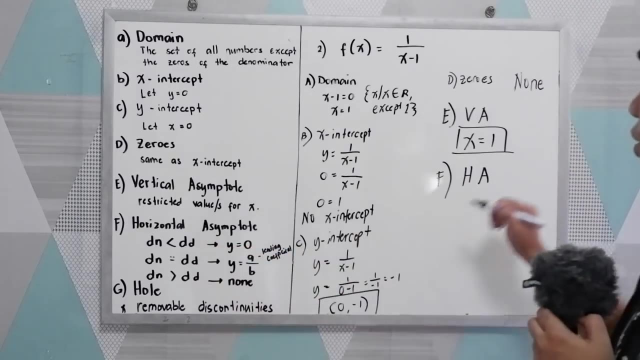 So we have here a degree of 1 in our denominator. That means the degree of the denominator is greater than the degree of the numerator. So we have our first condition: y is equal to 0.. And lastly, to find the whole, 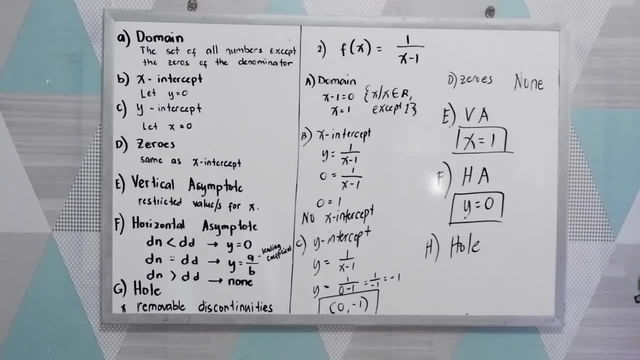 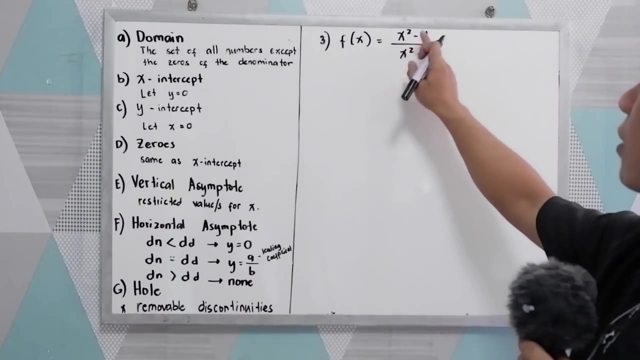 We don't have a common factor both in numerator and denominator. So for the whole, 9.. Simple as that. Now for number 3. M of x is equal to x squared minus 4, all over x squared minus 9.. 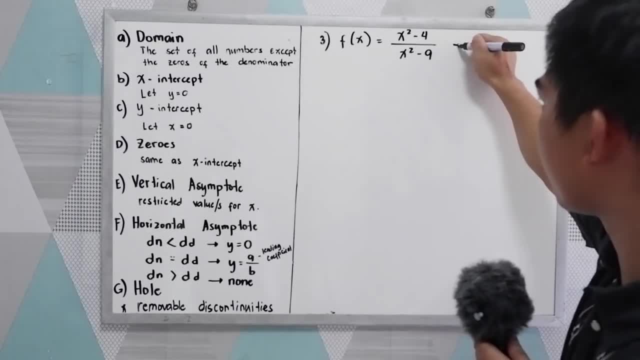 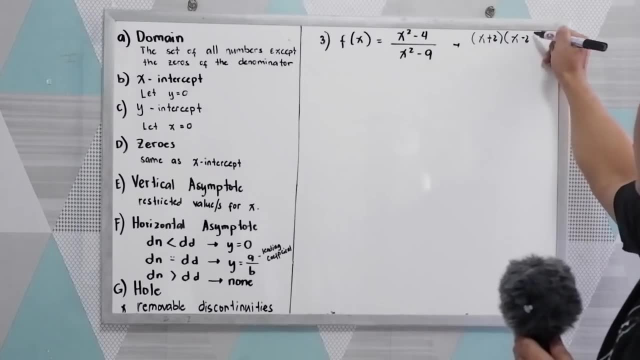 Okay, let us find first the factored form of our given In our numerator, that is x plus 2.. x minus 2.. And in our denominator we have x plus 3 and x minus 3, different of 2 squares. 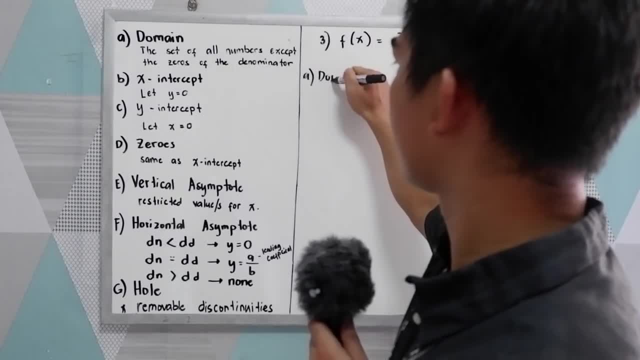 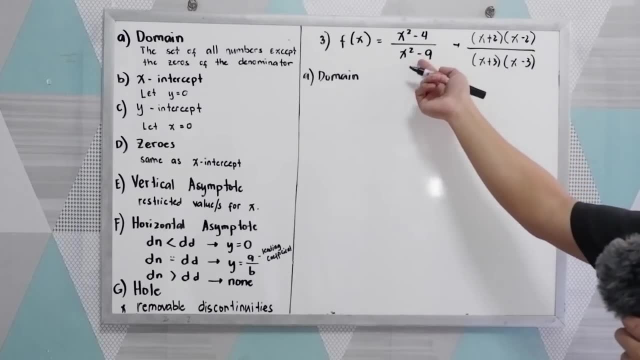 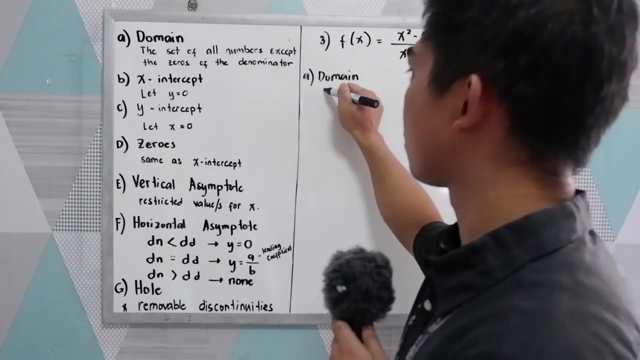 Now get the domain domain. Our denominator is x squared minus 9, that is the same as quantity x plus 3, times x minus 3.. So that is x plus 3 and x minus 3, equate to 0.. 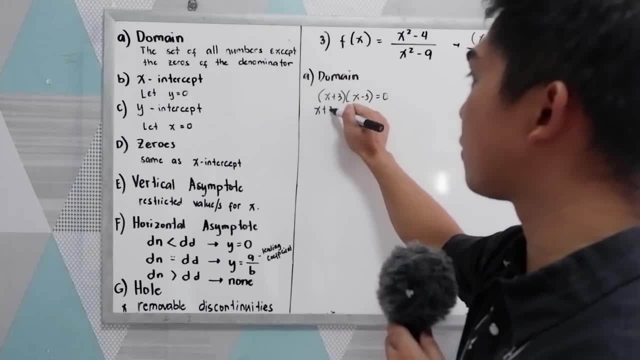 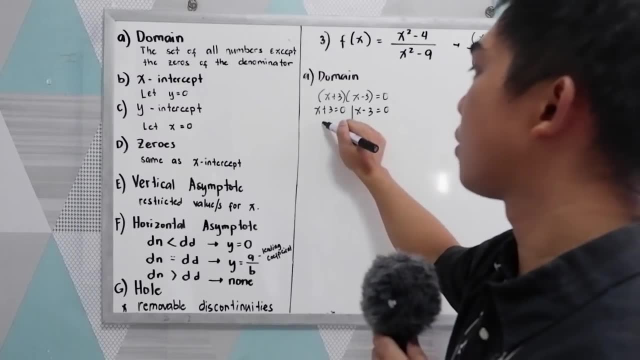 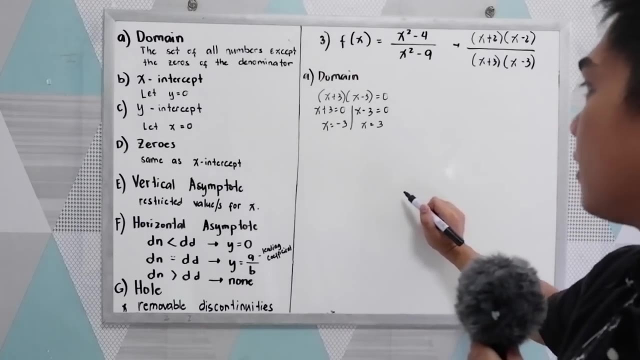 Now solve for x. We have: x plus 3 is equal to 0 and x minus 3 is equal to 0.. So we have: x is equal to negative 3 and x is equal to positive 3.. For our domain, x, such that x is equal to 0. 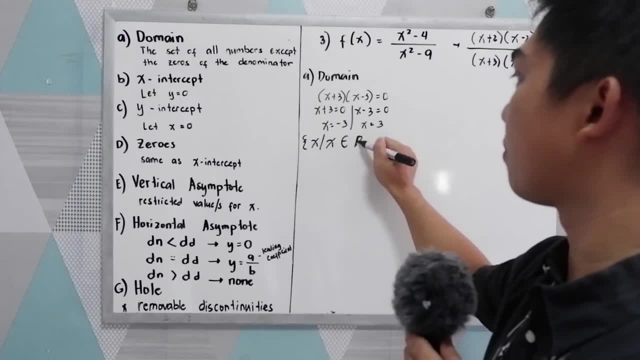 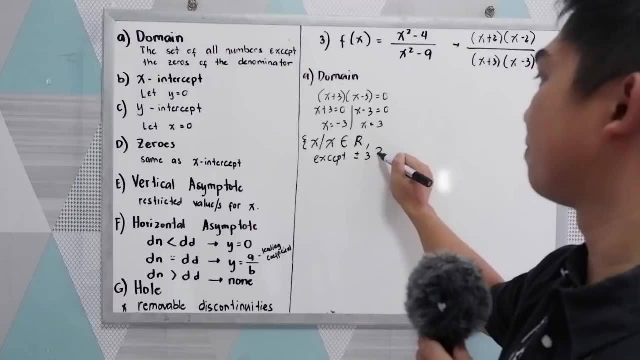 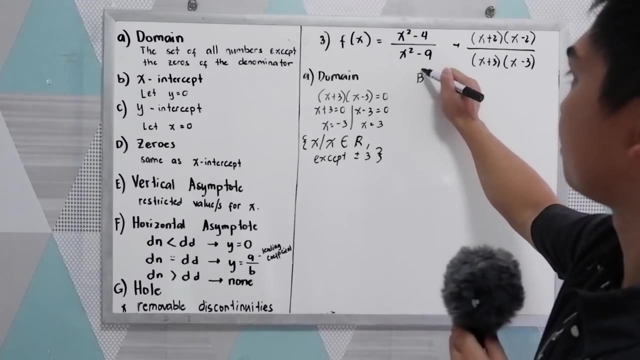 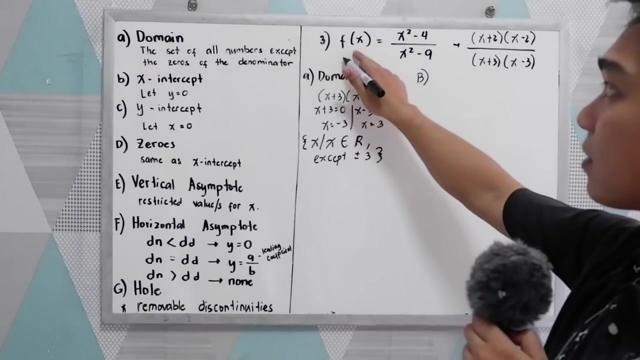 Okay, Okay, So x is an element of real numbers, except positive, negative, 3.. Okay, And for the x intercept letter B, let y be equal to 0. So M of x, that stands for our y. So 0 is equal to x squared minus 4.. 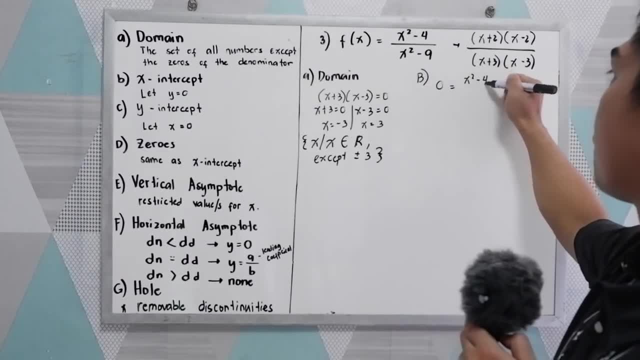 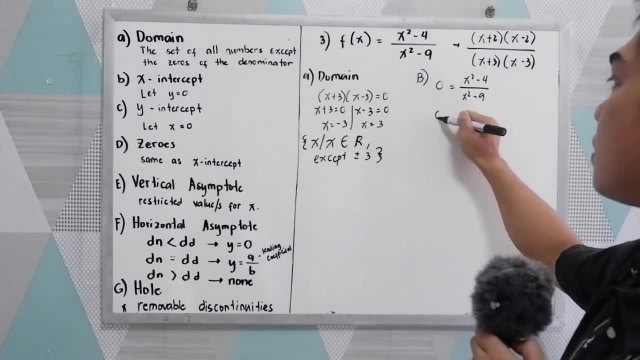 So y is equal to y minus 4.. So m of x is equal to m of y minus 4.. So y is equal to m of y minus 4.. So m of y is equal to m of y minus 4.. all over x squared minus 9, cross, multiply, we have 0 is equal to x squared. 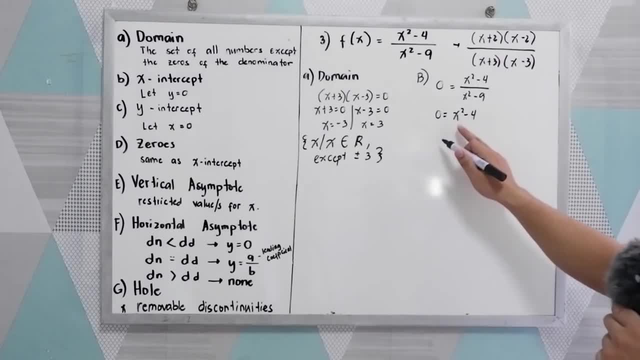 minus 4, get the factored form of x squared minus 9. so that is, 0 is equal to x squared minus 4. factors are x plus 2. x minus 2 now equate to 0. so x plus 2 is equal to 0. the other one, x minus 2, is equal to 0. so our x intercept you have. 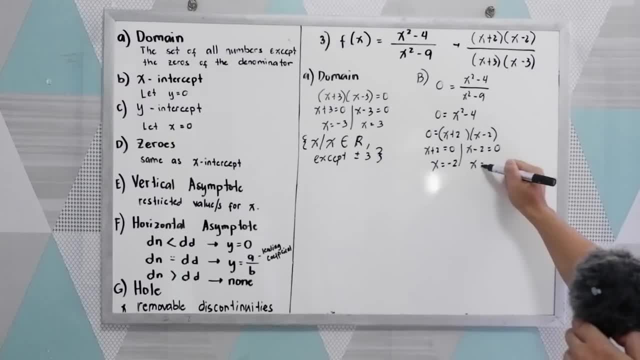 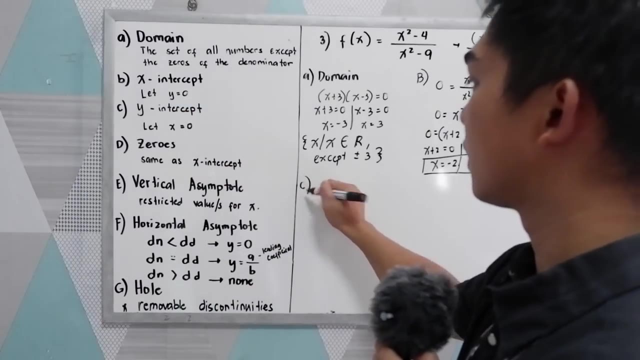 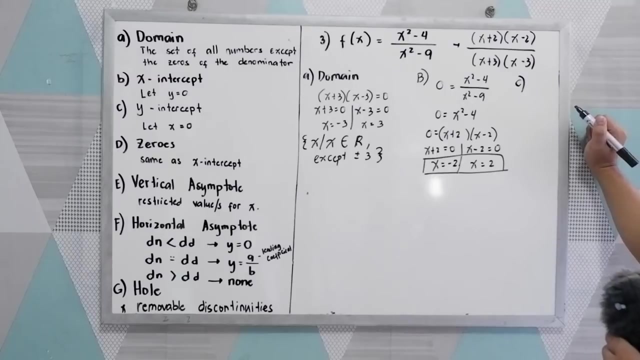 two values. we have negative 2 and positive. that is our tax interest. and letter C Y intercept. letter C Y intercept. let X be equal to zero, so in this case Y is equal to the. that X beats is zero. two zero squared minus four. all over zero squared minus. 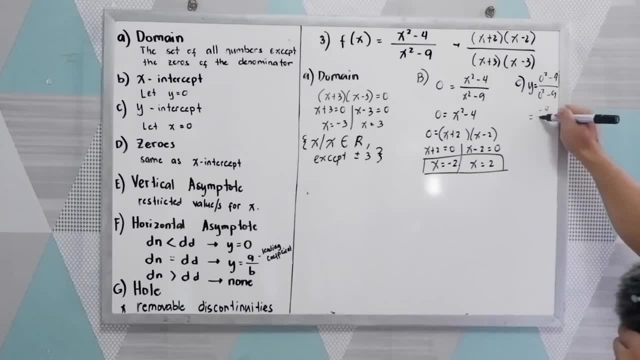 zero squared minus four, all over zero squared minus 4 is X minus zero. that is our X E Q E, X E Q E. I, let us see, does there? in this case we have root 9, so that is negative. 4 all over negative, 9 negative divided by negative. 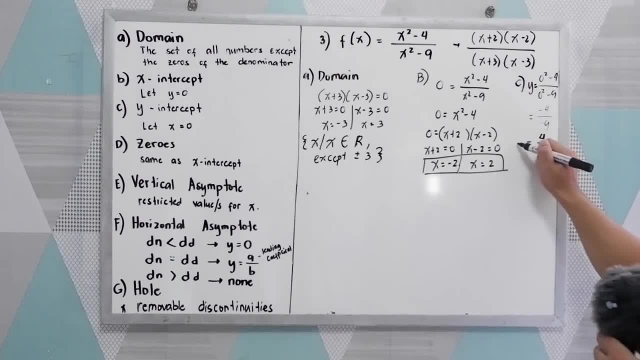 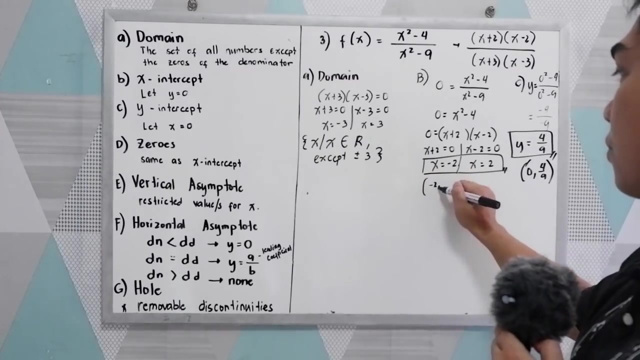 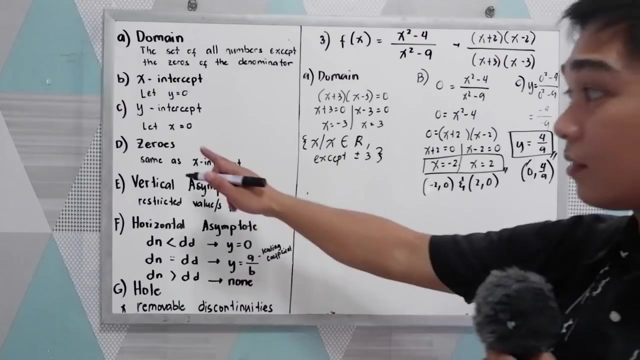 that is 4 over 9. so Y is equal to 4 over 9. so we can write this as 0, 4 over 9, so that you can easily plot the points. and for this one we have X is negative, 2, 0 and 2, 0. okay, now get the zeros letter D. 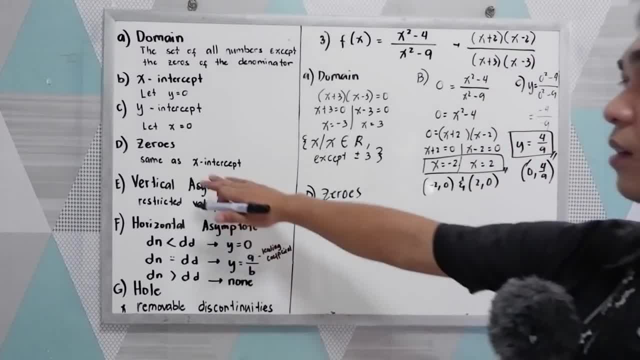 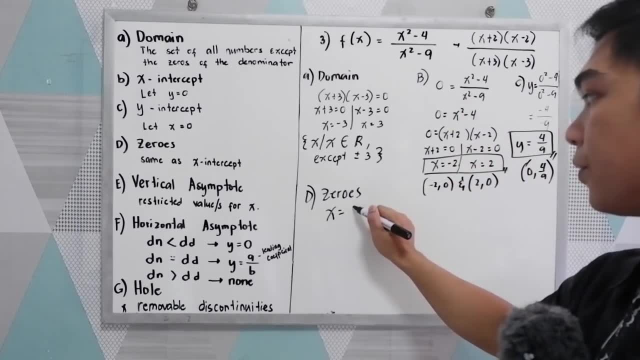 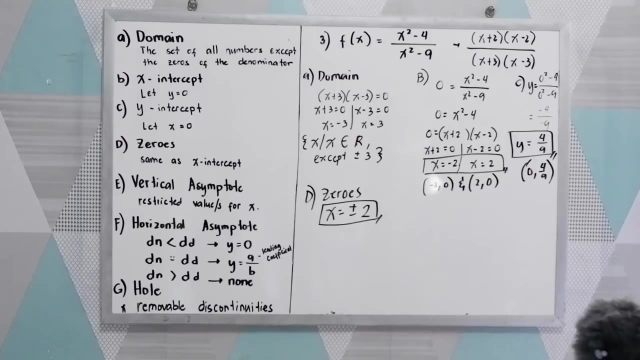 zeros. for the zeros same as the X intercept. so letter B: X intercept. so our zeros: X is equal to positive, negative. 2. give us X from positive moon. 2, Y from positive moon. 3. next letter E: vertical asymptote. for the vertical asymptote, according to our 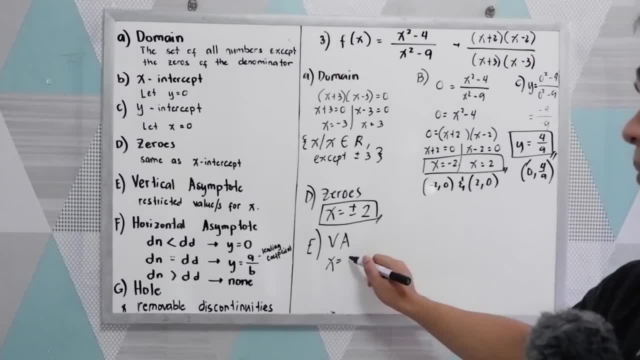 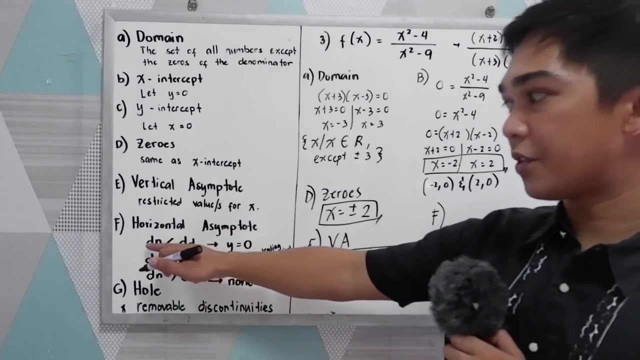 domain. our restrictive values are positive and negative 3 to negative 3.. Those are the vertical asymptotes And letter F, horizontal. So examine our condition. condition 1, if the degree of the numerator is less than the degree of the denominator. 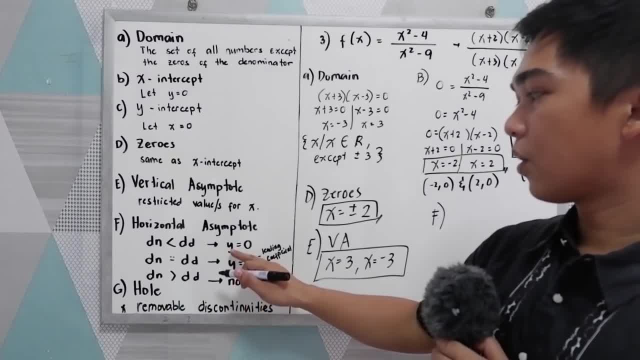 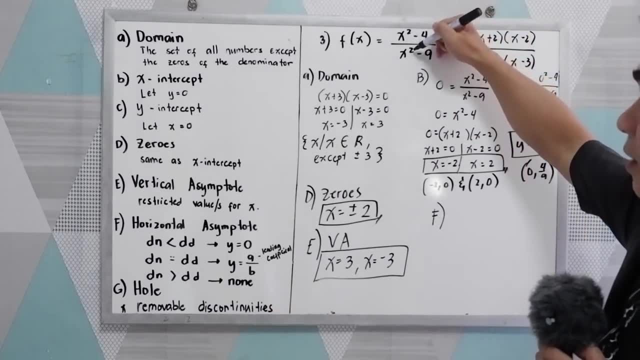 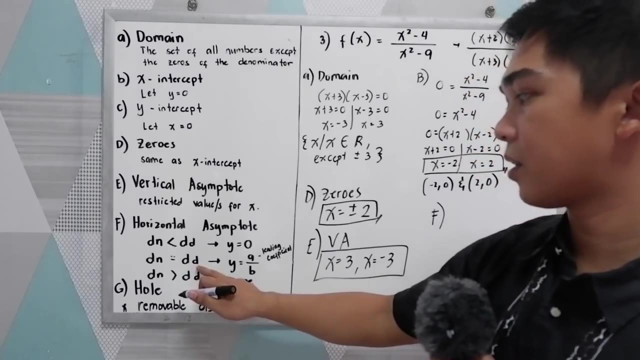 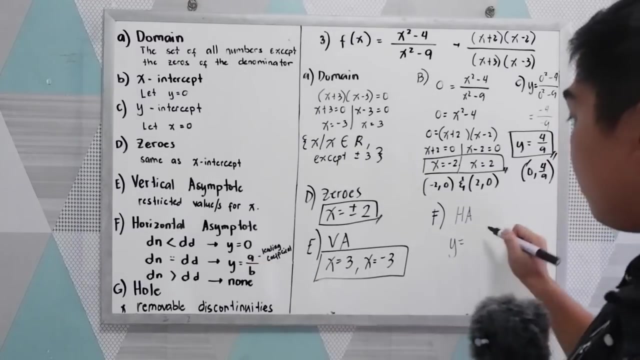 that is, y is equal to 0. So study our given. we have the same degree. So our degree of the numerator is equal to the degree of the denominator. So we're going to use: y is equal to a over b. 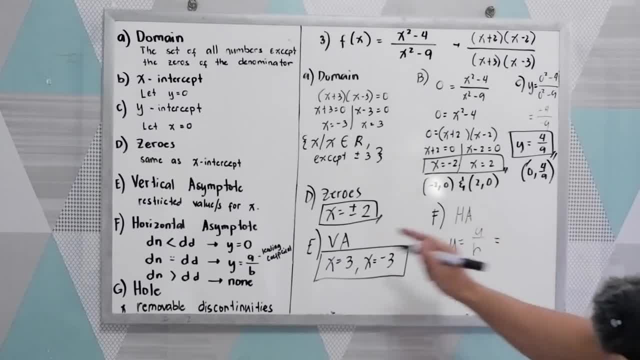 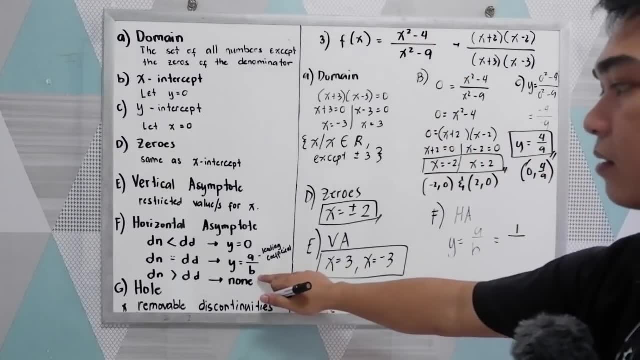 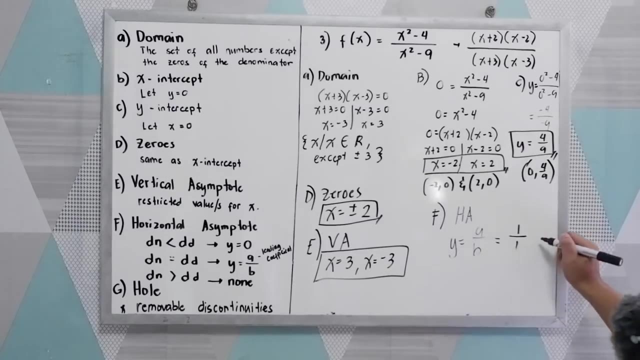 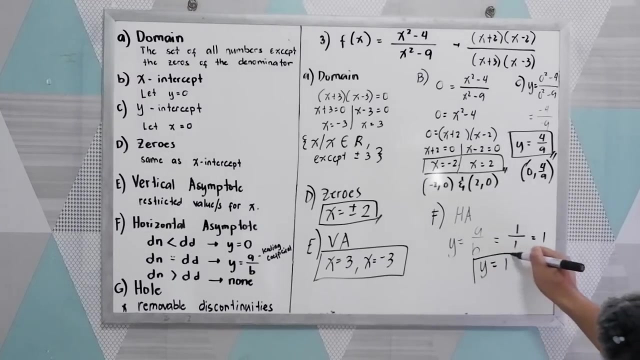 wherein a is the leading coefficient in the numerator- in this case you have one over- b is the leading coefficient in the denominator. we have also one, so one divided by one that is one. so our horizontal asymptote is: y is equal to 1 and our hole, as you can see in our fun third factor form, 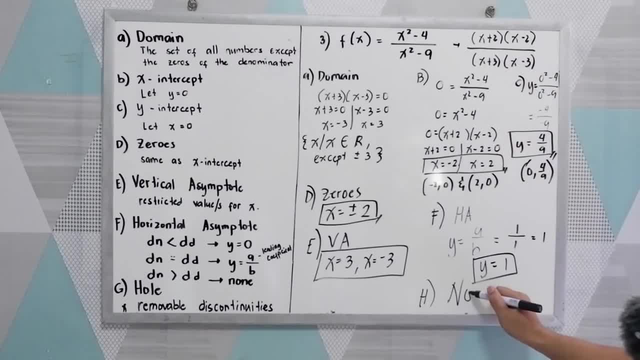 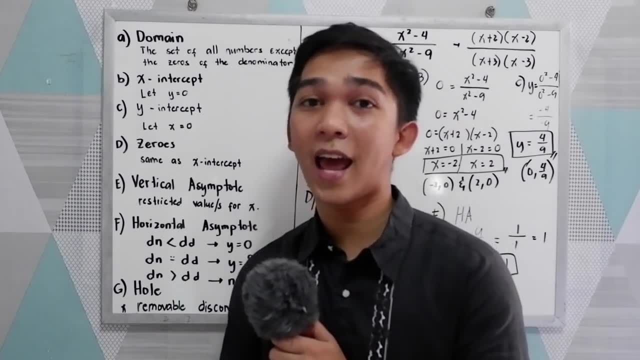 we don't have a common factor, so we don't have nine. i hope you understand the rational function and how to get a domain x intercept, y intercept the zeros, vertical asymptote, horizontal, and so again, you need to understand the state of the mind and how to get the domain x intercept. 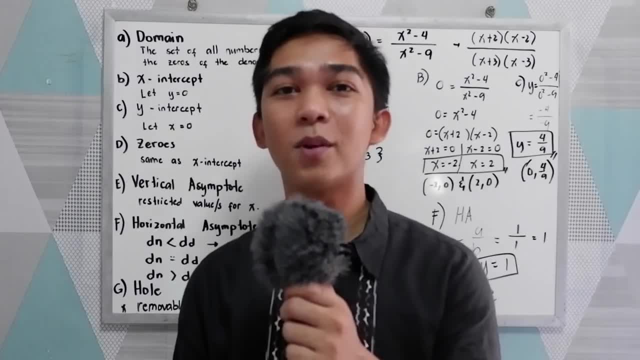 and i will tell you how to get the domain x intercept, y intercept, the zeros, vertical, the whole. Thank you for watching Senor Pablo TV.